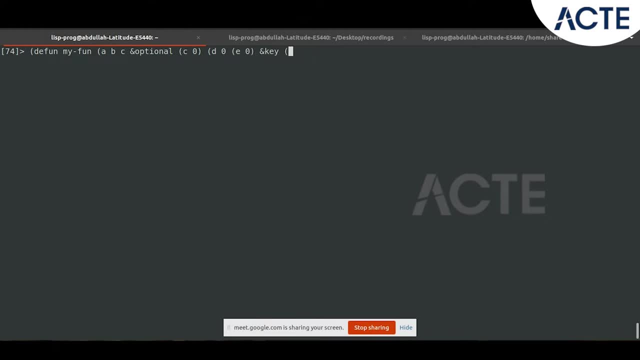 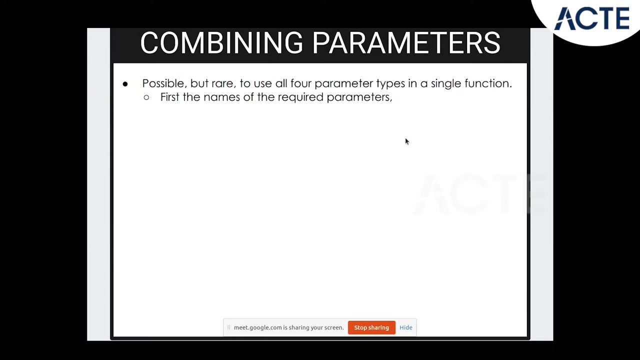 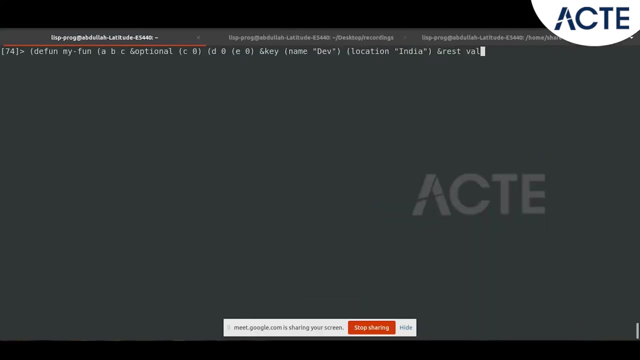 And then location, And we can then have ambus interest for all of the rest of these. So this is the sorry no. First the required parameters, then option, then parameter, finally the keyword, So you can put the keyword last. And why this is, you will have to see it later on. But this 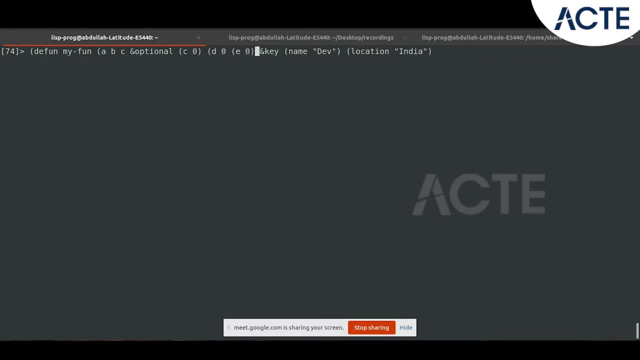 is the order. If you want to use all four, use it this way. And the reason why this will work is because the reason why it will work is because key you can- actually, you know, you can put it last. basically, You can put the rest and then you can put the keys in. 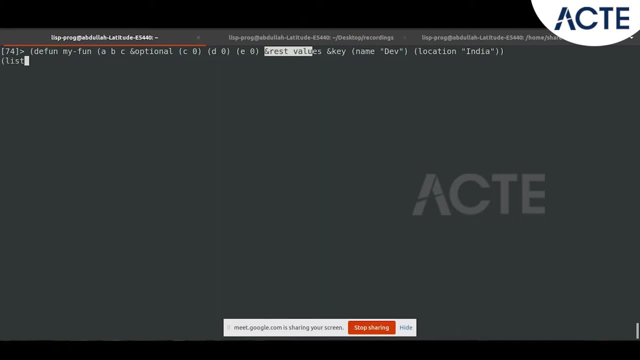 Okay, So I am just going to return a list, list plus of a, b, c, d, e. I can do this. Then I make a list of- I am putting values here which will be default binary if you do not. 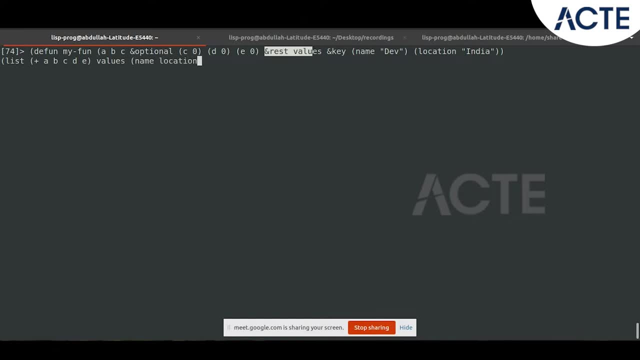 provide anything, And then name and then location, Just for, I mean for. so I need at least two parameters, Okay, Okay, Three, four, five. Yeah, I guess there is no way of you should be able to do default here. no, Why is it not? 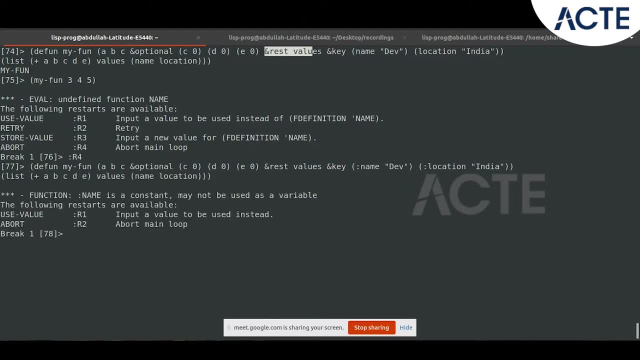 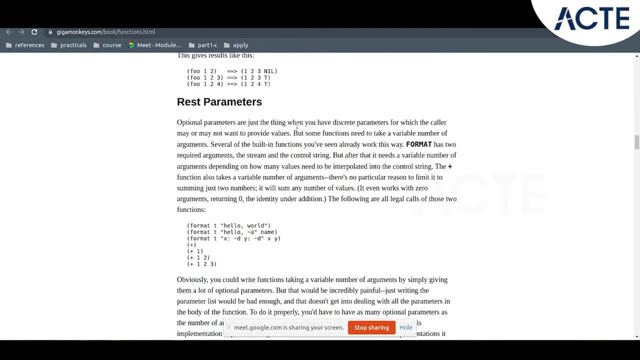 giving that? Do I need this key? I guess there is no default for keywords? Yeah, Actually there is no, So optional and the rest, of course you cannot give anything. The rest is basically whatever the user provides. Okay, But for keyword parameters. 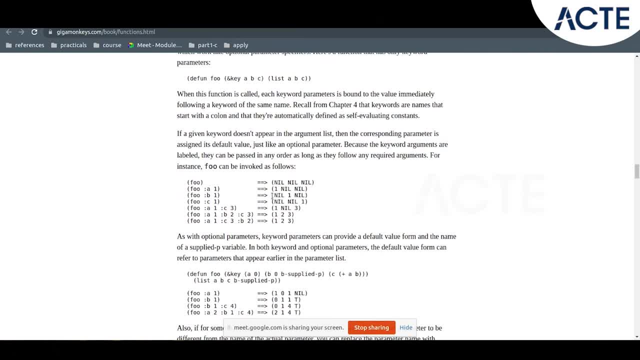 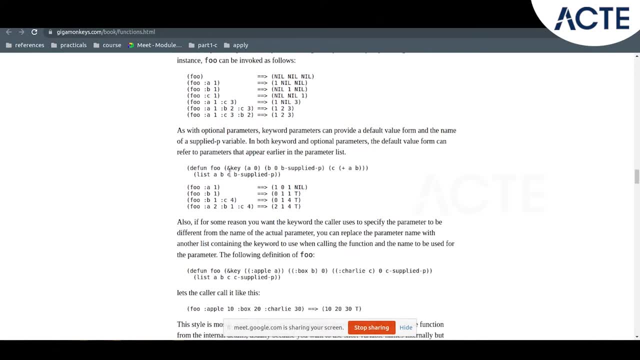 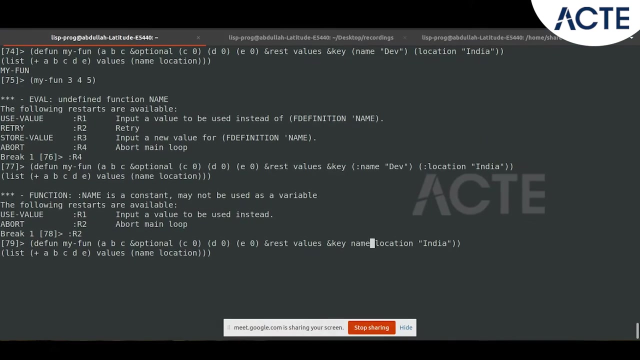 Okay, Okay, You should be able to do this, Right. Why is it not allowing me to do it? Okay, The? Okay, let us just try it out with the without giving default values. okay, or let us try out one default value. 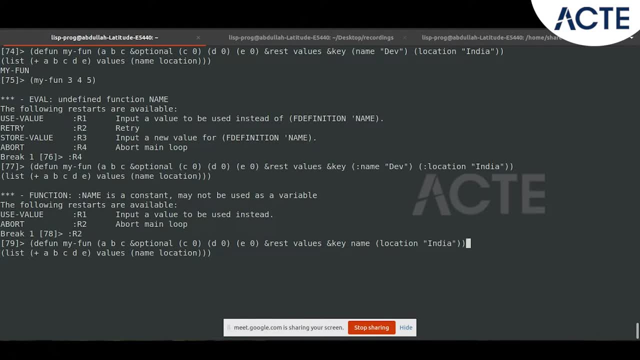 Yeah, okay, Sorry, that was the again parenthesis that I showed you. That was the parenthesis that I showed you. Let us see We should be able to give a name Names. They should be developed. Yeah, Don't know why they are not working. 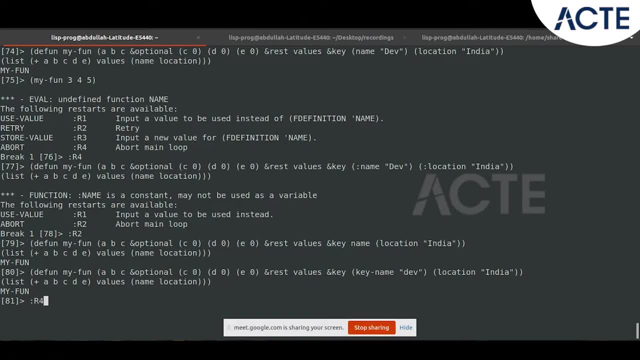 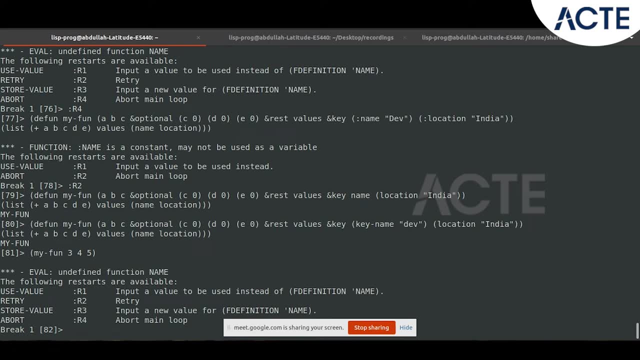 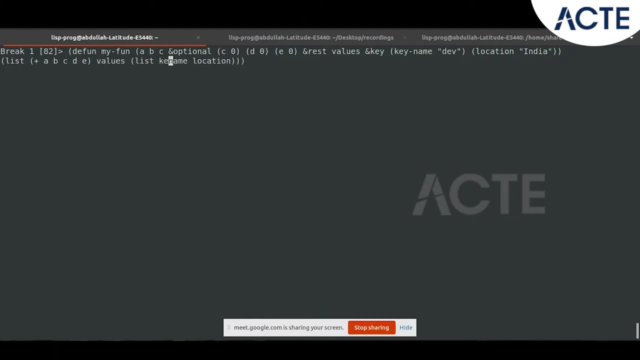 So this is the way to do it. Okay, My function, but you are O5.. Okay, The function name. Okay, Oh yeah, Sorry, this is. this is the issue. Okay, So, because because this became an S expression, so this was expecting a value or what I could. 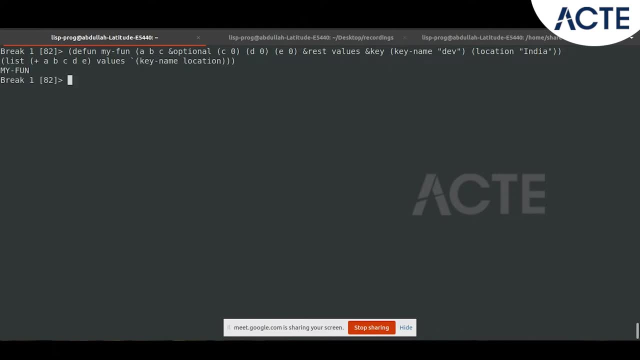 do is. I should have quoted it like this: Yeah, So quote. by the way, there are two ways of quoting it. One is the yeah, So yeah, this is not right, because I don't want a list. This is what I want. 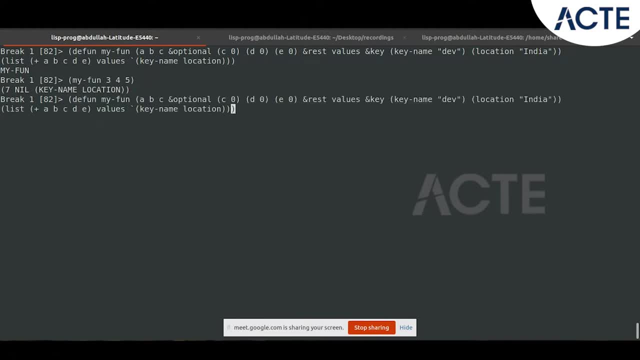 Okay, Now it makes sense, Right? So this is the way it works. So my my fun for three, four, five, If I put in anything, if I put up to let us say one, two and three, all of these are. 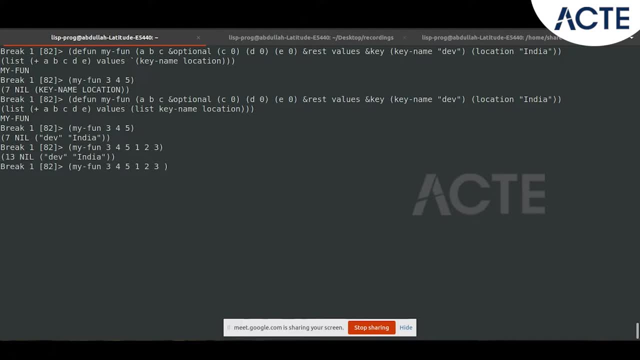 optional. They will get summed up. So if I move ahead with the 131,, 179, this will come into values. Yeah, So that is a. it is not. actually there is interest values. Okay, Again, that is so. this is the issue with the combining things. but actually he said 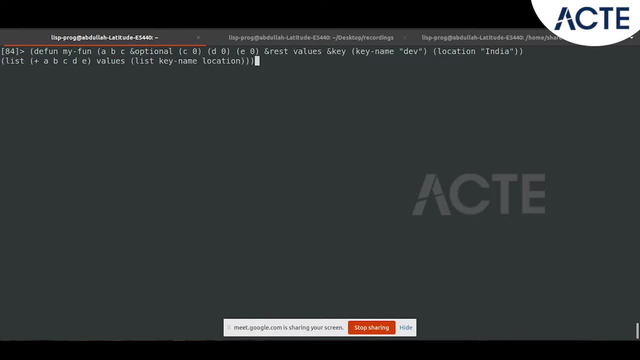 that it should not be an issue Anyway. so let us just do without the key. So I hope you get the issue. what the problems that we have when we combine, combine things. Okay, This is the problem that you can face. 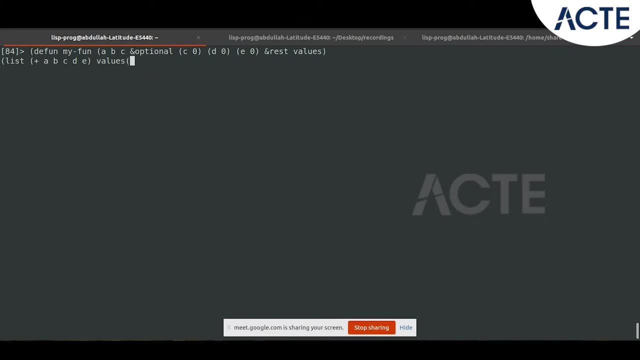 So when you try it out, you will know what is the, the challenges that are you need to face here. So with this thing we can actually you can see that you know. so first you will match the, so I am combining optional with the rest. 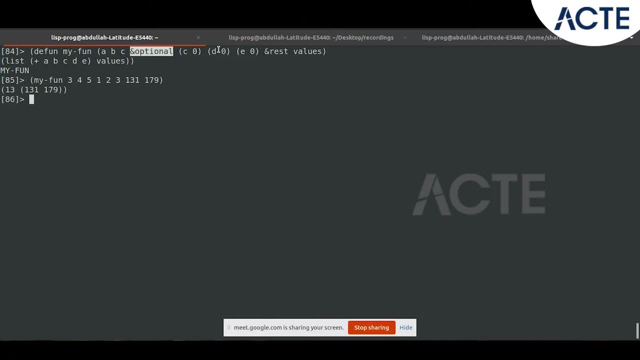 Okay, So today we will not go much more into this. I will have a look at it again and I will come back with this. So we have combined three parameters: Okay, Required, optional and rest. So this is. we can also have keyword symbols, but we have to be take care of how it works. 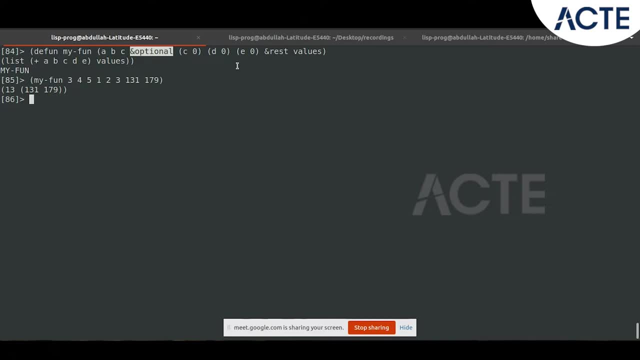 actually. So we will not do that right now because we do not have time for that, But we can see that we are combining required, optional and rest values, Okay, So when you do that, the first three are, of course, required. 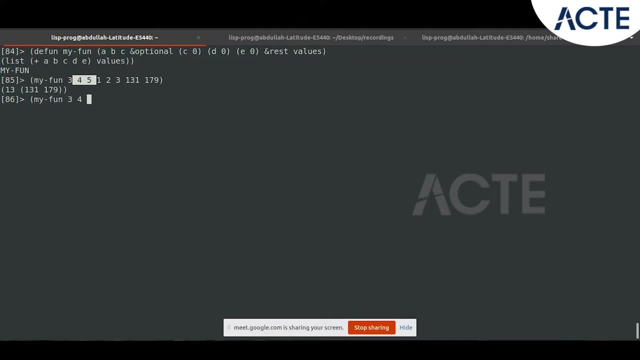 If I do less than three, it will not work. Okay, If I have less than three parameters, it will not work. So that is the required parameters. It requires you to type in at least three, but once you type in three, it is going to. 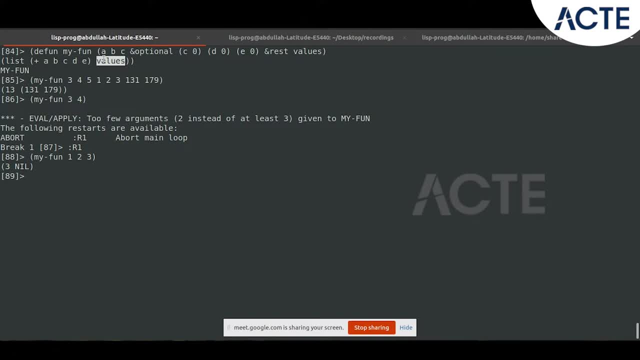 work, Okay. Only thing: the values will be nil. All right, The values. you will not have anything there, So it will be nil, Okay. And yeah, optional will be also will be zero. It is the default values. 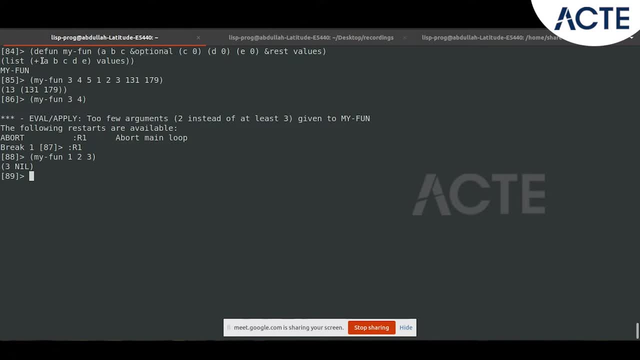 If it was not zero, it would have thrown error because I am adding all of that, Okay, Okay, So I am adding all of them here. So I definitely need a default value And if, by default, if you do not put a default, then the default is nil. 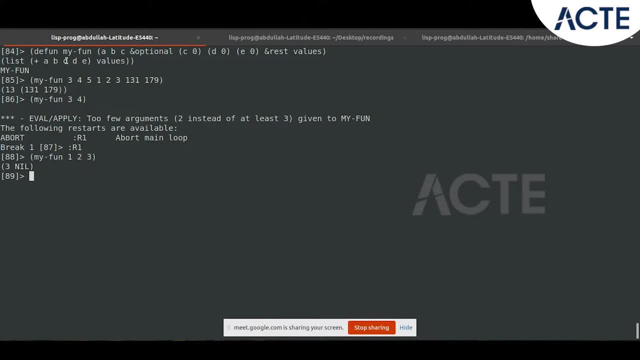 That will not be suitable here. You cannot put it into this CDE thing. Oh, but there are two Cs, by the way, So that is another issue with the code, So that it seems to be taking the first one. Yeah, 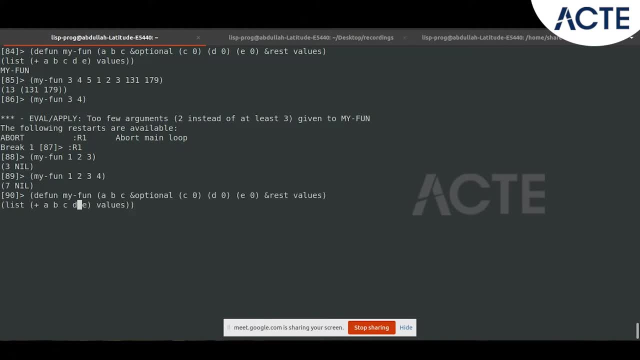 It seems to be taking the first one, So you have to also make sure that you know you name the variables properly. Okay, Okay, You cannot. if you overwrite it, this will get hidden. That will be yeah. So the flexibility does not give you the. you know these things. you have to do it on. 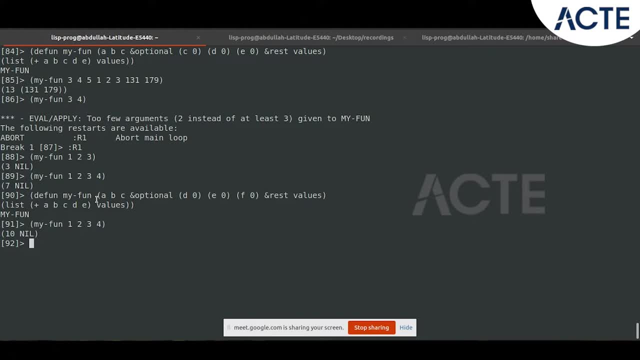 your own. You have to make sure that all your variables are unique, and so on. So with combining required optional and rest, we saw like what happens here. This is quite clear. actually, This is something that is clear because you can see what is happening. 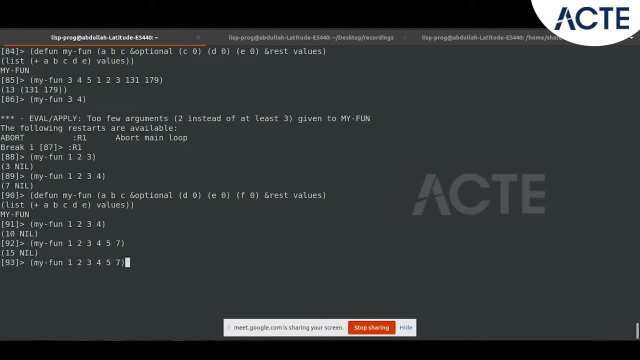 I mean, you can reason with it, So it is not so difficult to understand it. So what will happen here is: this will happen, Okay. So what will happen here is basically: but you can see the options that you have. 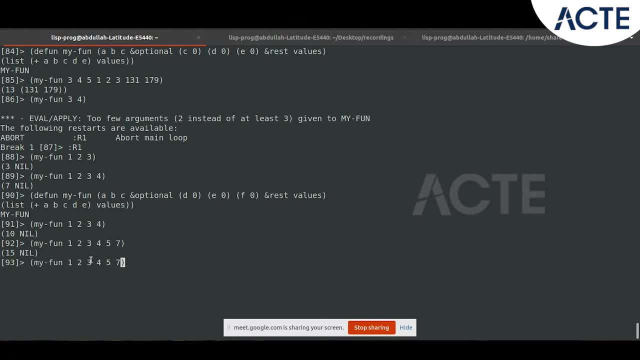 So first the ABC is mapped to 1,, 2 and 3. Since you have DEF, you get mapped to this here. Then- and this was nil so far- Then you can add in parameters. Okay, This will go into. it will get caught into the values. 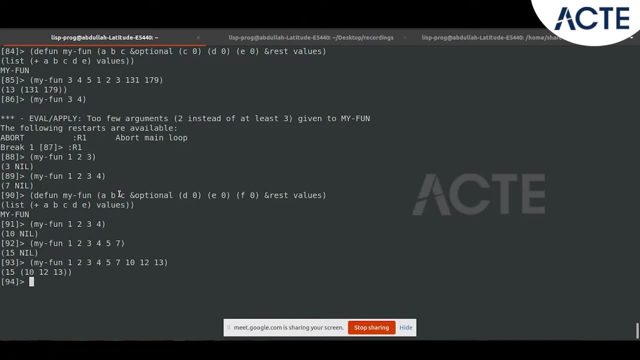 Have these things here. So this is how you can combine. So we have combined required optional and rest. Okay, And there are some you know very fine things you can look at and do it So we can take it up later. 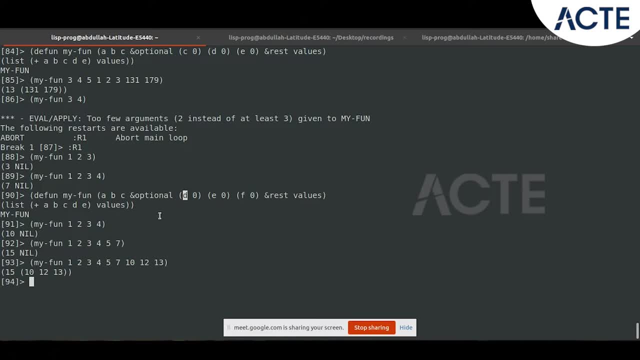 So, as you saw right this, when you start combining the parameters it can get a little bit involved, So we can look at it later. But basically you can see that we can combining three parameters: required, optional and rest. 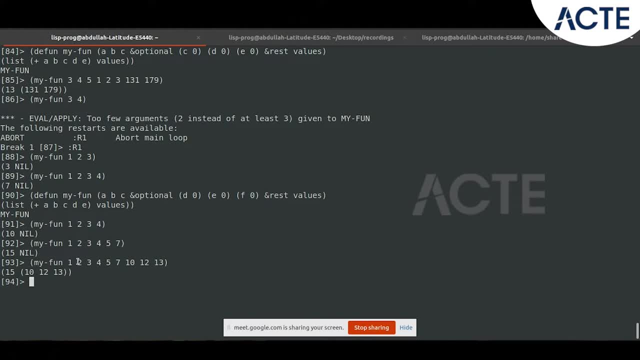 gives you some amount of flexibility in the way to and how we can go about using things. Okay, And I will give you some exercise on this, So we will look at it later on. Now let us move on to the exercise lecture today. 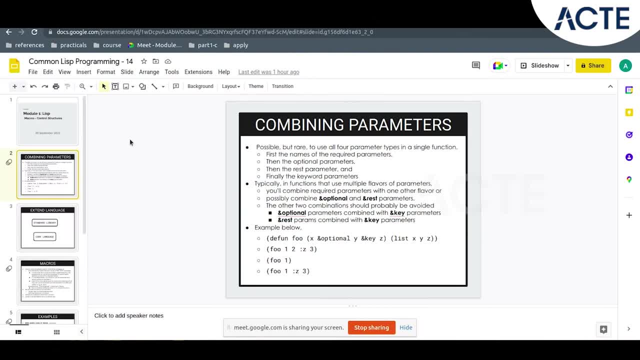 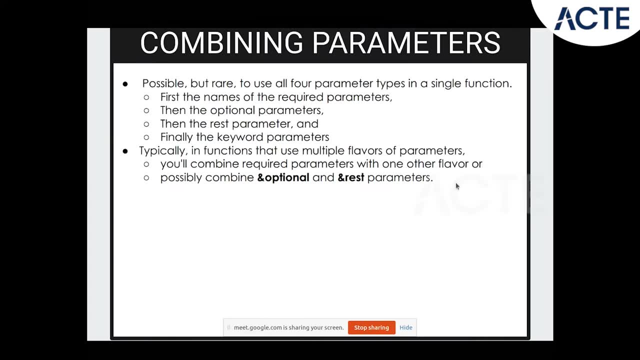 So for today we will be covering. main objective for today is to cover macros. Okay, To go into macros, So what I will have? the idea is: okay, let us. so this is what I meant here. 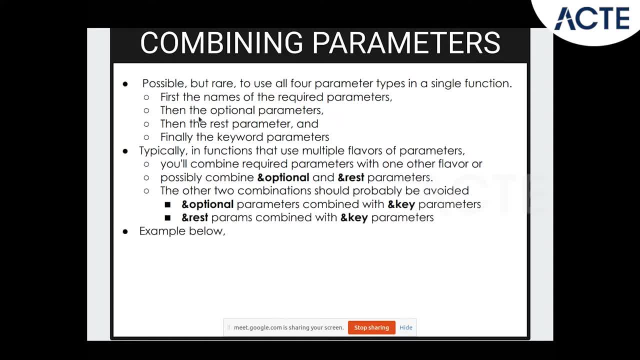 So typically. so you can actually combine all four of them, but this is very rare. Okay, It is possible, but rare. So I showed you how to. we combined optional, required optional and rest. So typically what happens is that you can combine all four of them. 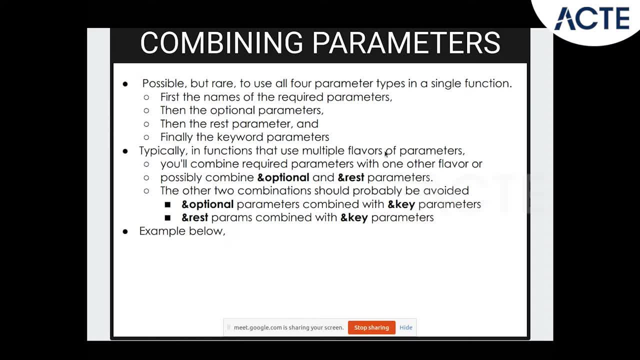 But this is very rare. So typically what happens is that in functions you have that use multiple flavors, You will either combine required with one more, one other flavor. So that is why I told you, can, you know, have a look at it. 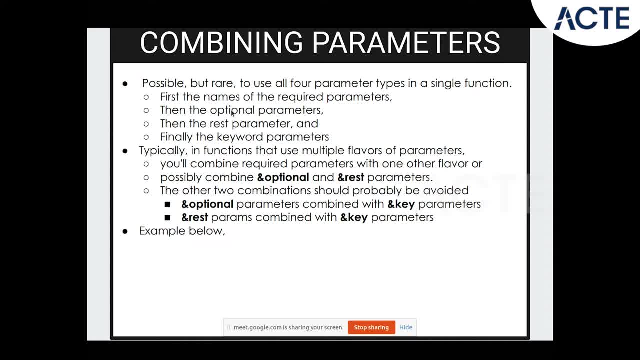 And at least, even if you get food at one, each of them individually, you will be good to go. I mean, you will have some idea, you will be able to do some amount of, you know, substantial amount of programming, some amount of things you can do. 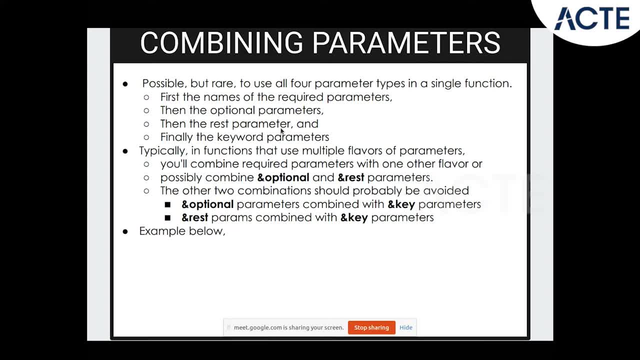 See, for example, rest. you can actually have arbitrary. You can allow the rest. You can allow the user to define arbitrary arguments. Optional allows you to have between discrete number of things, between n and n plus m, some number of parameters your function can have. 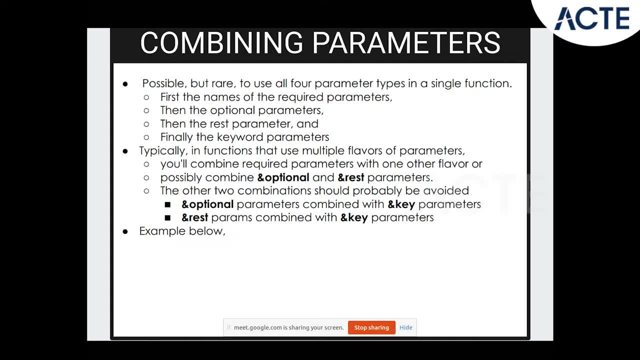 So, even if you use one of them, one additional parameter, if you are able to understand how it works, it helps you to write functions and to understand existing functions. Then another way is to combine optional and rest parameters, which is what we did just. 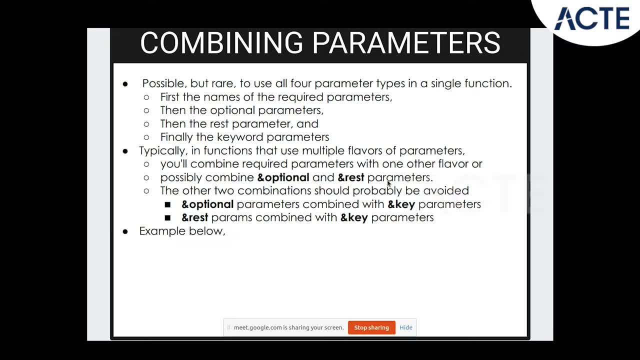 now, Right, If you can do that itself, we will have, We will be able to do a lot of things with it- Optional and rest And, in fact, some exercises I will give you on this, and you know you can, yeah, with. 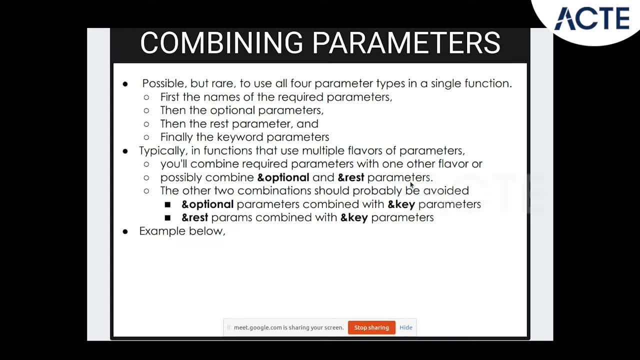 this, you can do a lot of things Right. The other two combinations- you think you probably avoid it: Optional and key and rest and key. So this you will. you have it explained in the book So people who are interested can go through it. 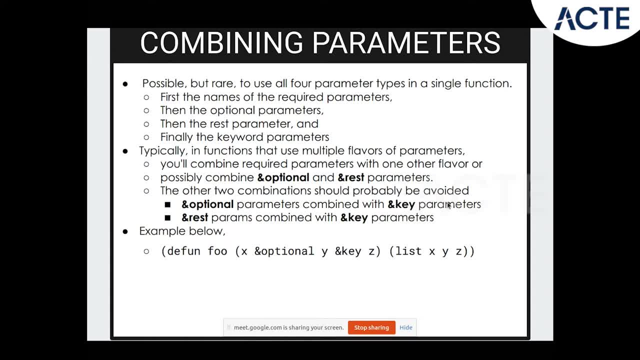 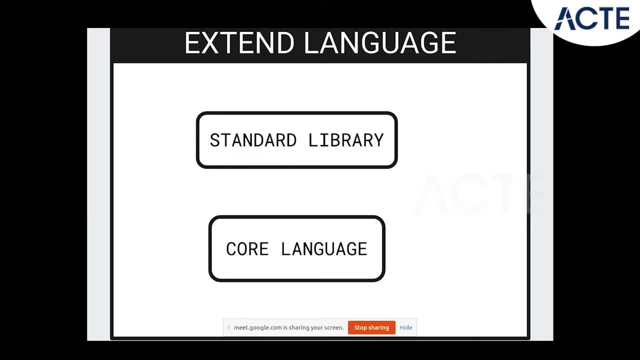 And maybe later, if I have time, I will take this up. So I will just keep this, Okay. So example is why it's become difficult. Okay, So you can skip this for now and we will move on to the next thing. 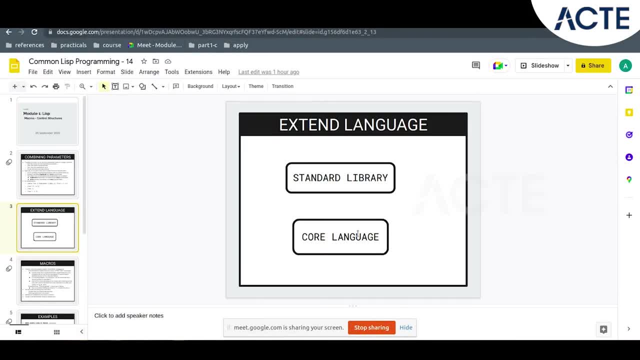 Extending a language Right. When you extend the language, there are two things. One is the core language. What does your language support in terms of low level things that have to be implemented? This is for language designers- Okay, People who design languages. 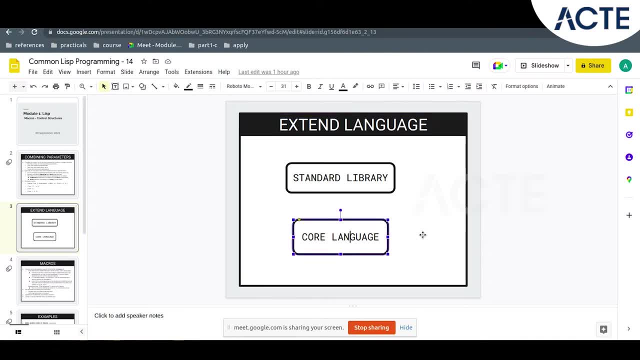 What does your core language consist of? What are the constructs that are core to your language? Okay, And once you have those core constructs, you usually build up a library of things on top of that That will help you to give you basic features. 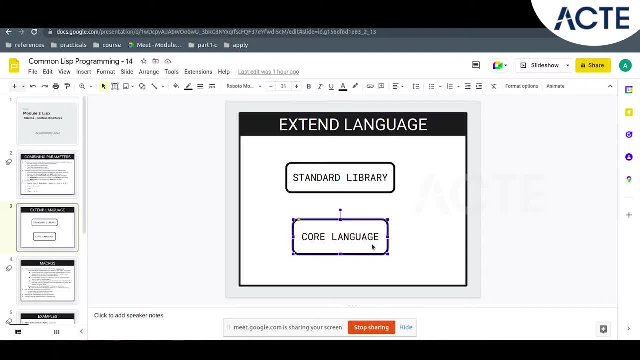 So your language is not just a core language. It's usually a core language in the standard library, like C or other languages. So in the language design you have this option. you can make your core language very small, And you know. 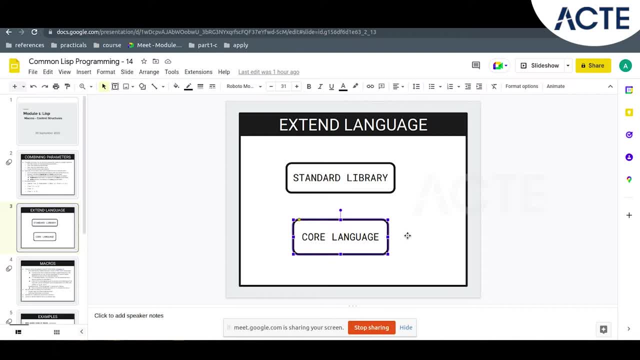 You can put everything in the standard library. The advantage of having a standard library is implementing the language becomes. one of the advantages is that implementing the language becomes easier If you want to port it from one architecture to another. say 64 bit to 32, I mean 32 bit. 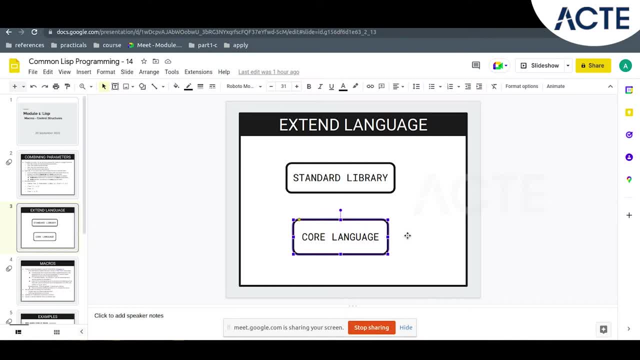 to 64 bit Or you want to, you know, implement in another architecture. All you have to do is you have to implement those core features. Once those core features are implemented, you can then take care of- I mean- the rest. 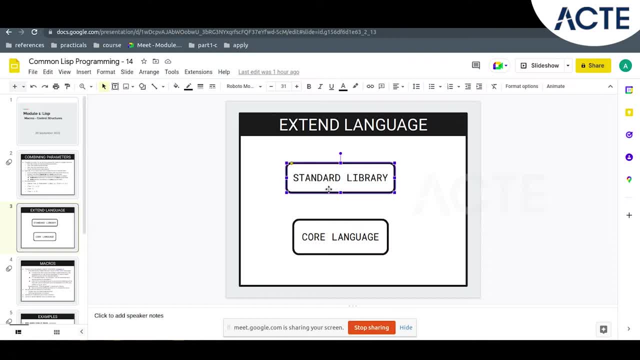 of the things will. the standard library will build in the language that you are using. Okay, That's what you are compiling to. All right, So if it is C, the standard library is written in C, like sorting, like arithmetic precision. 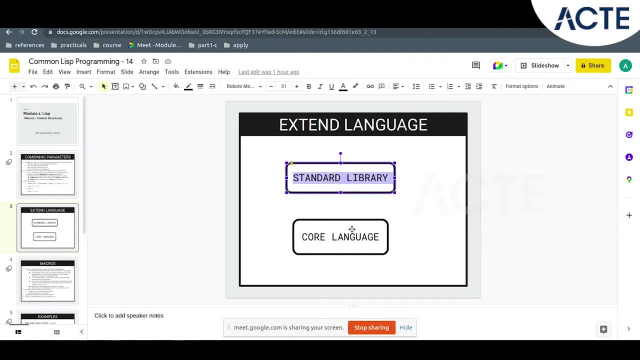 some amount of features are available, All right. So if you shrink, you can, so the users have these. I mean language designers have this option of either expanding the core language, And if you expand the core language it becomes difficult to port it to different systems. 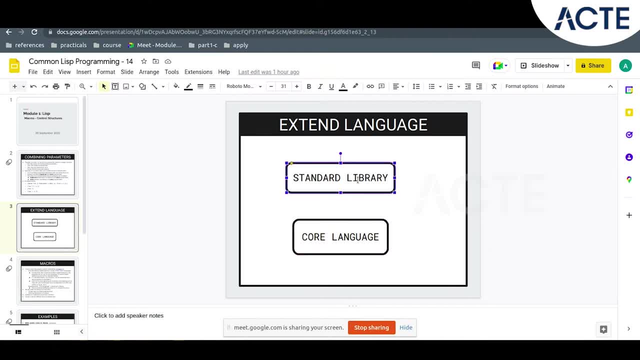 Or you shrink the core language and allow your library to run. So if you want your library to be arbitrary so that you know, arbitrary in the sense you put all the features into the library so that it is easier to port things. 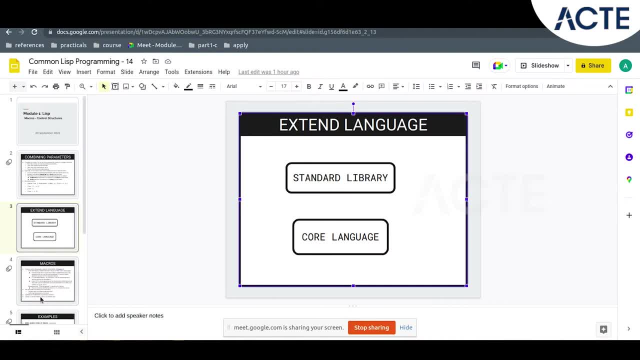 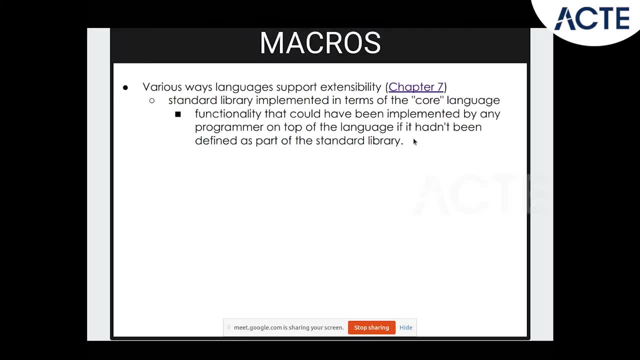 So one. this is one advantage of having an extensible language. So that is what is mentioned here. So macros is the approach, is the means by which, is one of the major means by which Lisp allows you to extend your language. 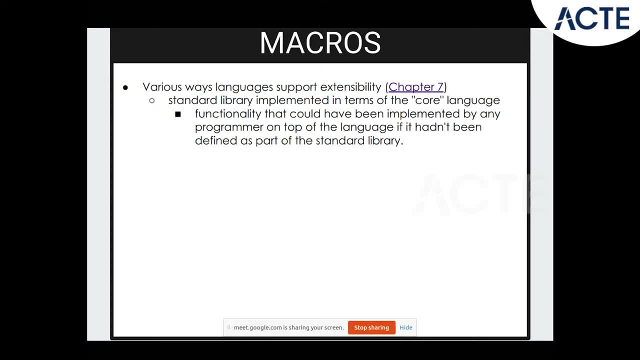 The core things are very small in Lisp- Not very small, but not very large either. Okay, They have a very small footprint, So it is easy to, and it gives you this macros option which allows you to extend the language. 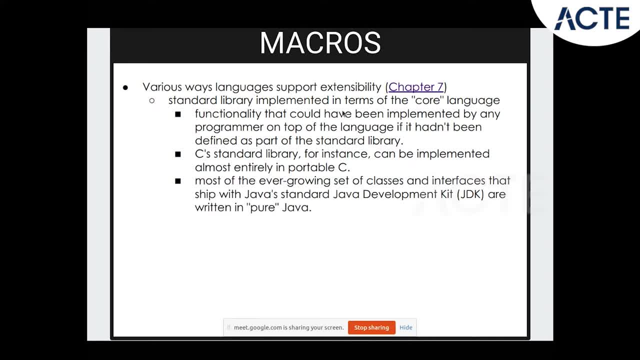 Okay, This is one way of extension. So this is one specific way of extension, which is for Lisp, And Lisp uses this macros a lot. All right, So what happens here is standard libraries in the core language. what I mentioned just. 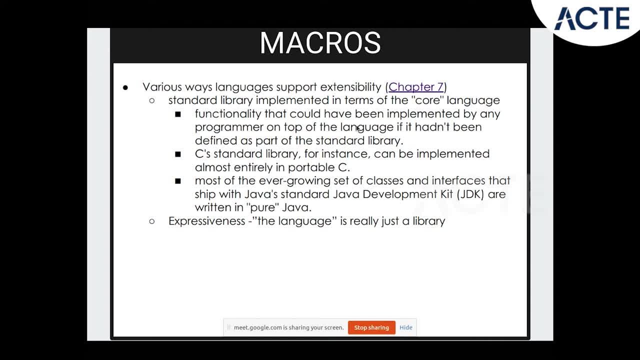 now. So this is the standard library- is something that could have been implemented by any programmer in top of the language itself. So the C language now, if it is a C language, the standard library functions could be implemented by any programmer on that language itself. 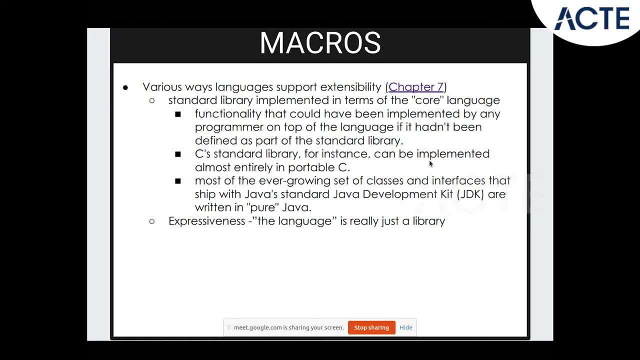 Okay, All right, So C standard library is can be implemented almost entirely in portable C, So there may be some other constructs that are mixed in, but basically it is essentially C. Okay, So C. you do not have to go into the low level programming. 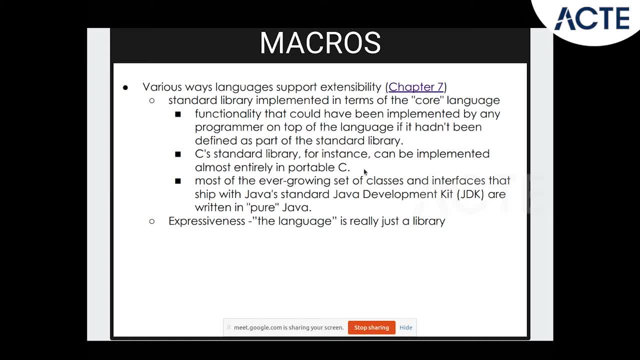 You do not have to do anything bit fiddling or whatever, in that You let the. somebody has to do the implementation. but once you are done with the implementation of the core features, you can always add in the standard library, Right? 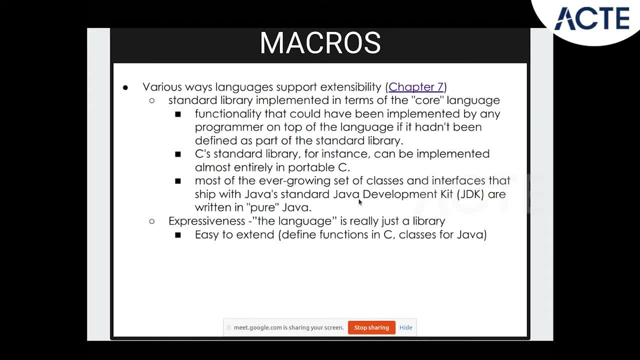 So, and JDK also has this same feature. Okay, So we have a lot of classes that sit with the JDK standard Java classes, which are basically pure Java, So it helps you to port it to various architectures and various environments. 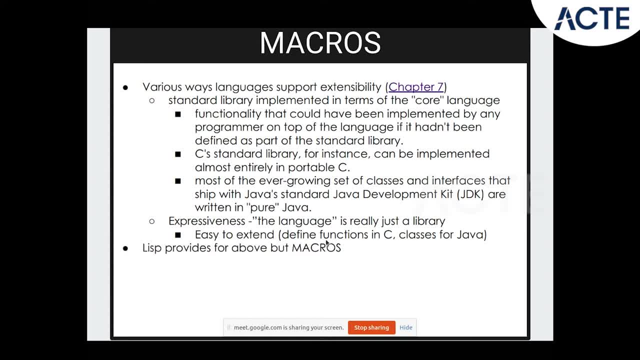 All right, And expressiveness is just a library- Okay. So what has happened, is it? Lisp also allows you to do this, Okay, But it has something extra for macros, All right, So it allows you to create new functional abstractions. 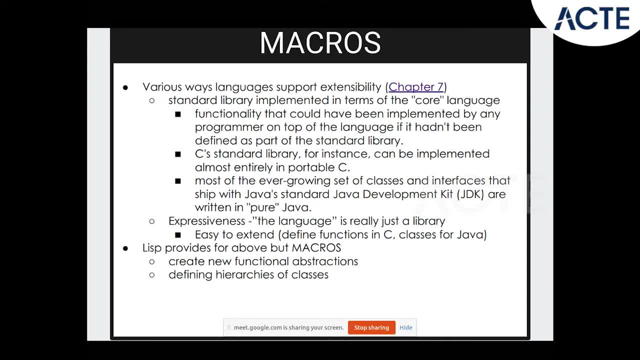 It defines hierarchy of classes and gives you macros in Lisp are very different from very- how do you say that? very powerful and very much, much more useful Then compared to other. it is not really other macros. what you have seen is quite different. 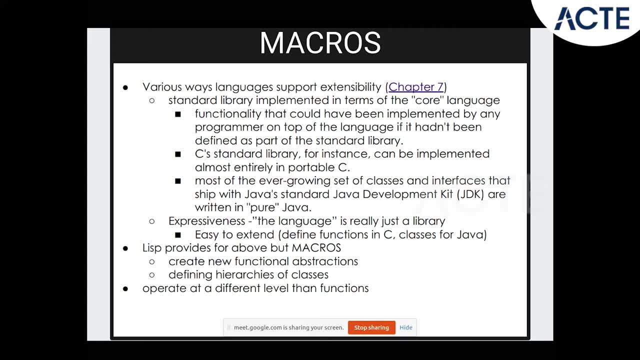 Okay. It is much more flexible and much more powerful, And that is the reason that we have used this to do a lot of things. There are a lot of things, So, in fact, we will have a look at it in the next slide. 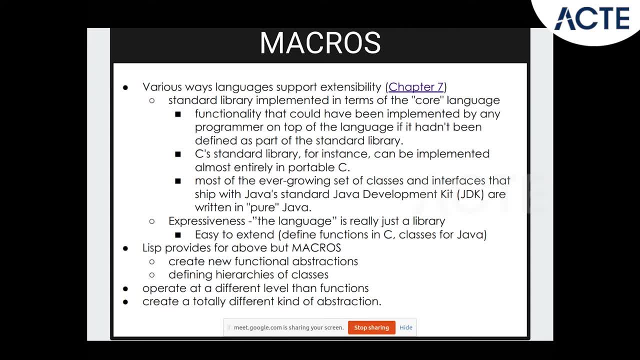 So it gives you a totally different kind of abstraction. Okay, So it is all about you know abstracting things out. This is not really whether you can do it or you cannot do it. It is like how you go about doing it. 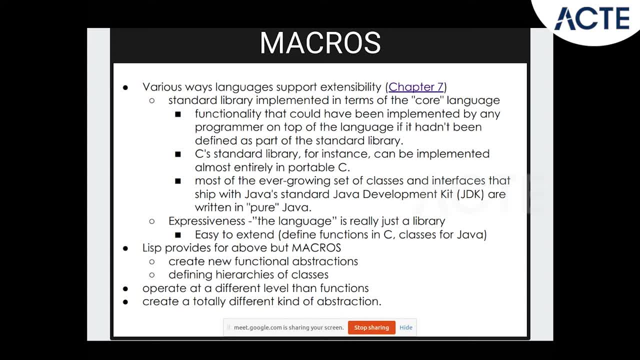 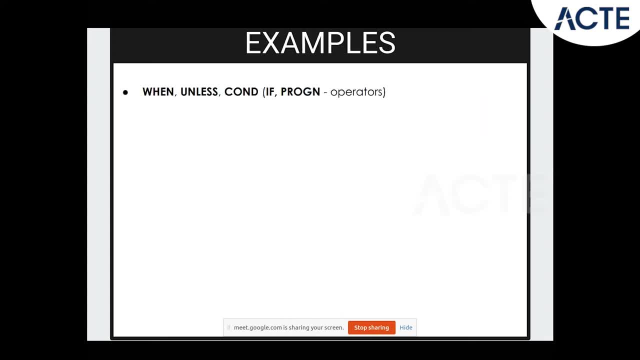 So this functional abstraction that we saw and kind of the features of the language help you to write macros to do a lot of things. Okay, And examples for that we have. So this is the control structures. Okay, So we have when, unless can't. 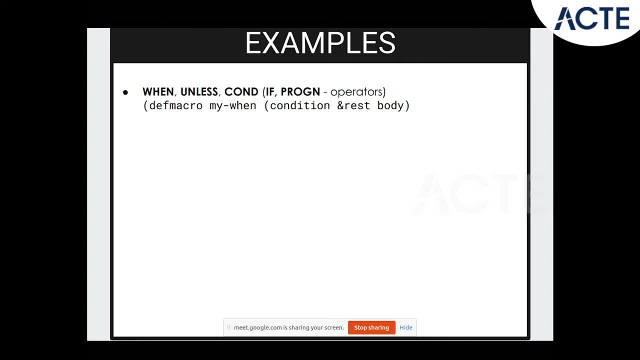 Okay, I will now go into this and I will let you know what this when is, what is the motivation for that? And there are other things. So this Boolean operators, Okay, So another. So I will just give you an overview of it. 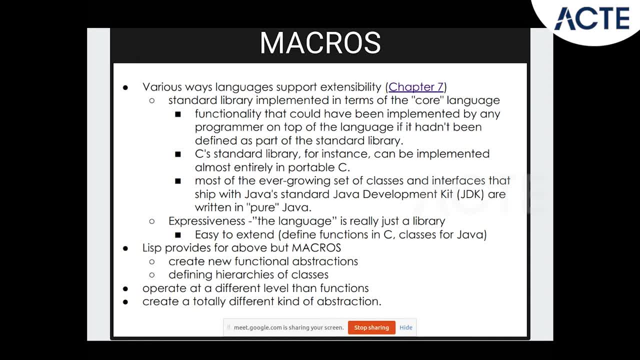 What all you can do with the macros. All of these are macros, by the way. All right, So macros is something that to, at a very high level, a very short summary of what it does. It is basically. it does not. this is basically. it is meant to be a. it is code that generates. 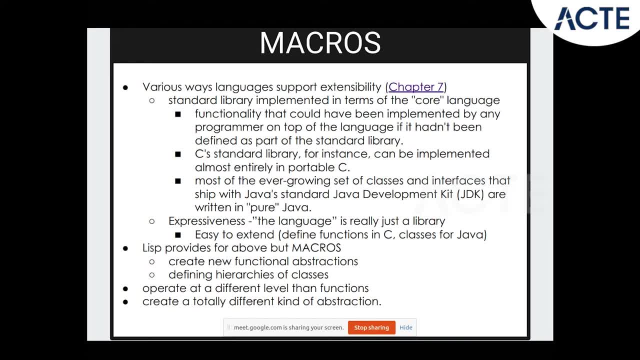 code. basically, Okay, At the end your macro will generate a. at the bottom level it will only be a function call and a special operator form. All right, You can. but you as a programmer can write your code in in as a macro and that macro. 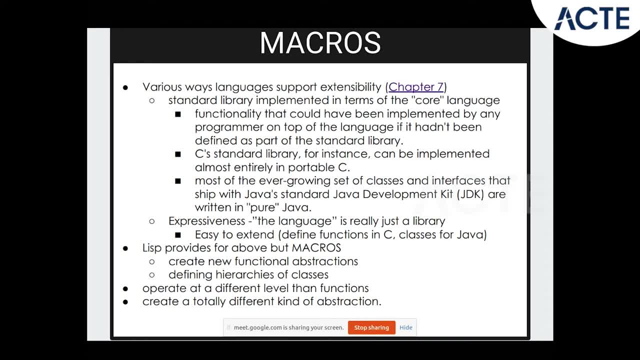 will get expanded at run time. It will get expanded at compile time and at run time you will not have that macro. that definition that you gave will not be there. It will just not be there. It will be expanded down to the low level constructs. 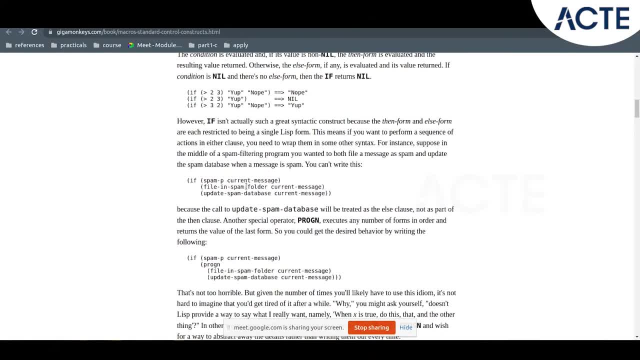 That is what a macro does. So this definition, as you see it, is basically any function. So I do not know if there are Intrinsic functions or if functions are, so functions itself will have. how will they be translated into? 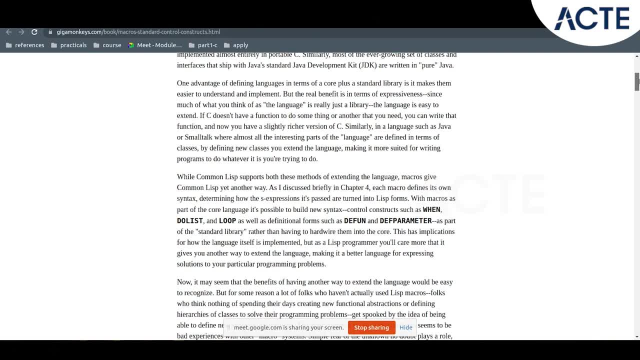 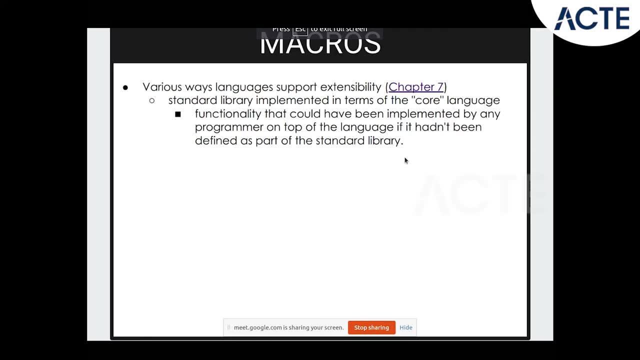 Okay, Yeah, So let us just keep it like this. Okay, Basically, what we have is: we will look into the details later on, So details are not relevant right now, because what macros does is we have two other forms. 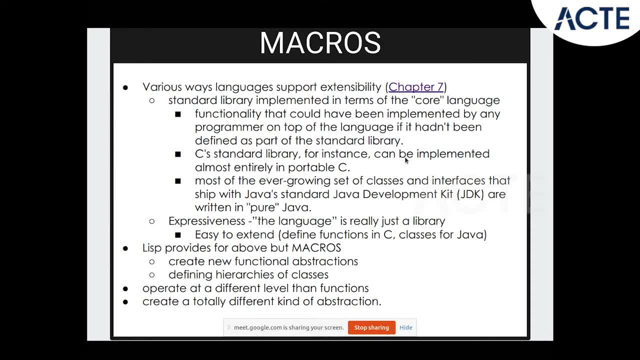 Right, We have function forms and special forms. All right, We have a functional form and a special form. So, special operators, special operator form. Macros is something that you can use as a programmer to write your code at a very high level. 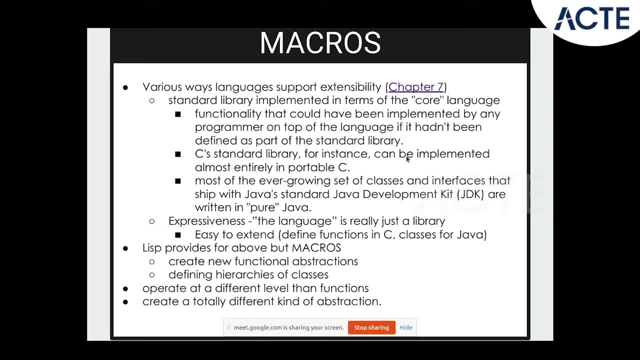 Okay, And at the low level there is some very. there are 25 special operators in common list. All right, There are only 25 special operators, which is not very small, but it is not very useful. It is just enough for a list. 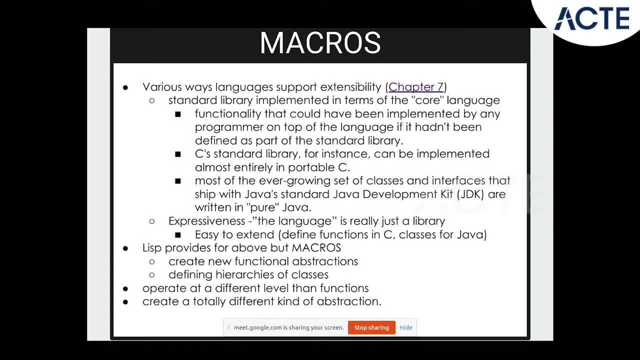 And everything else is either macro or a function call form. So this macro, it will get translated into a function, It will get translated into a. at compile time it will get translated into when you compile the program. the macro will be removed, will be translated. 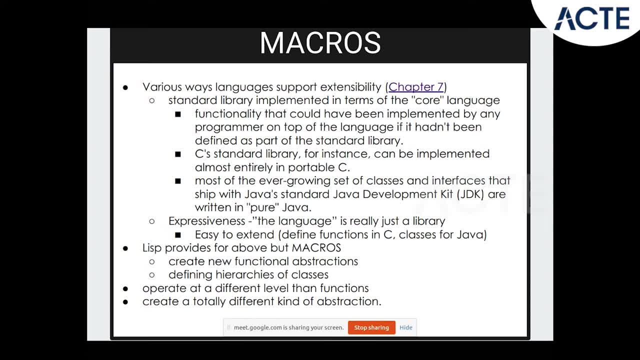 It is like compiling. All right, When you compile, what do you do? You take a source language and you translate into target language. So what will the list compiler do? It will take a macro and it will plug in the definition that it translates into. 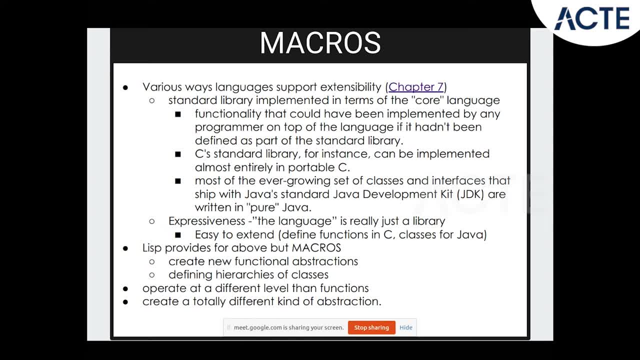 And the thing that it replaces the macro with will be only consisting of: at the end- Okay, Because there are many iterations that it can go into- But at the end, after it is done compiling completely, after it has expanded all the forms, the only thing that will be remaining in that executable or the code that it is. 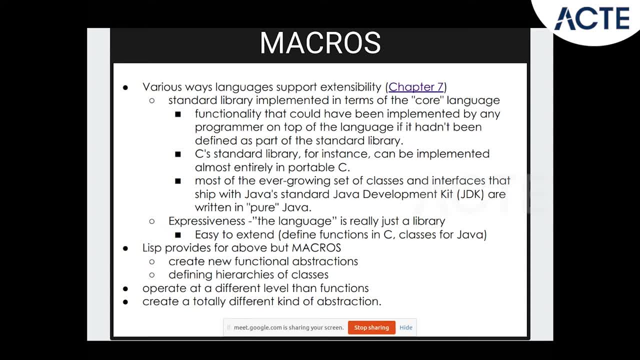 going to run is it will be a function call form or a special operator form? It has to be one of this, All right, And we will look at. I mean, if you go in depth, we will know what exactly how it is. 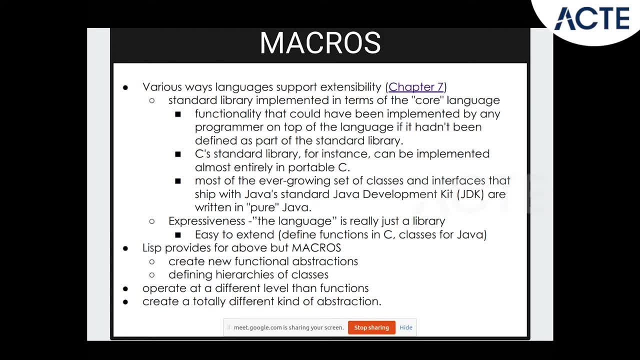 getting translated and the mappings. But it is enough to at this moment. I think it is enough to say that Your macro will be eliminated in the final thing. that is going to run. Okay, And this happens for when you compile it. 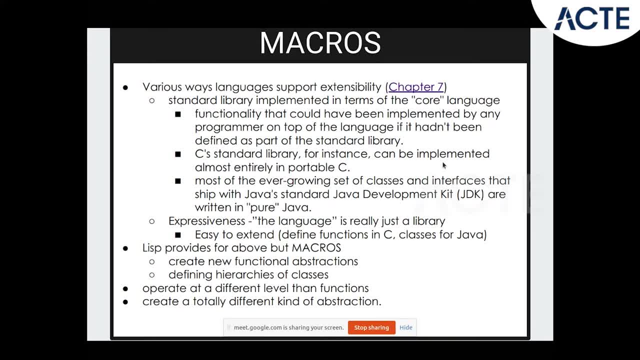 As I said, Lisp has both. You can do both- compiling as well as interpreting. But this is this example is more relevant for when you compile a thing, Okay, And for interpreting. what it does is in the redevelop print loop. it is only interpreting. 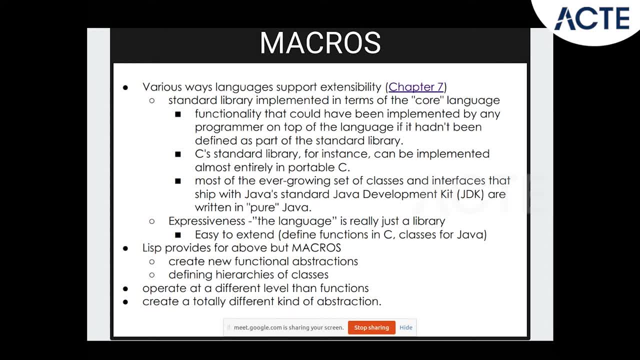 Okay, So there is some amount of overlap In the sense that How it reads this. if it has to interpret it, how it reads this thing, It has to actually expand it. But it will expand on the fly And there are options for it if it is an interpreter. 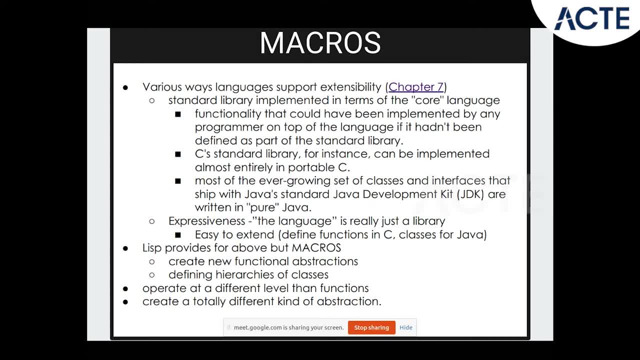 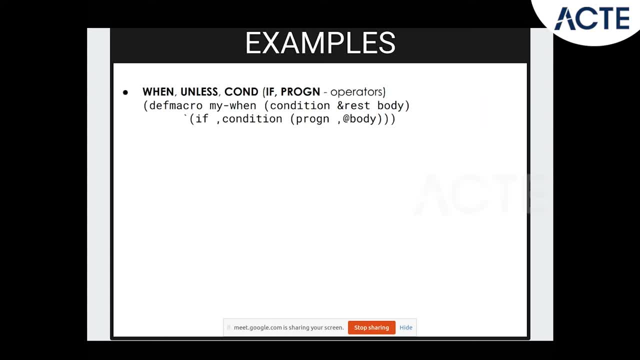 Okay, So there are many ways in which it will go about expanding a form, But, at the end of the day, the actual code that you run finally will not have any macro. That is the concept of a macro. So- and these are examples- 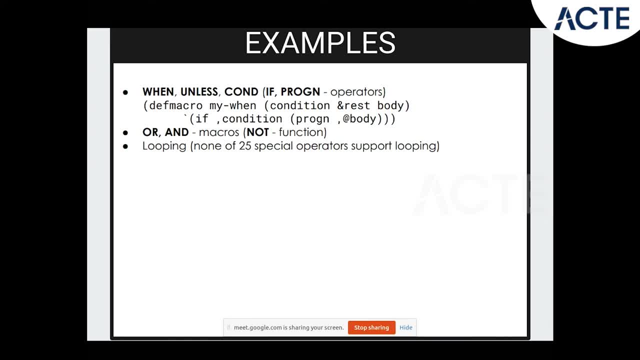 Okay, Control structures. these are. All of them are control structures, And yeah. So one example we have here, And you have also Boolean things Like or and and. Okay, Macros, Whereas not is a function, All right. 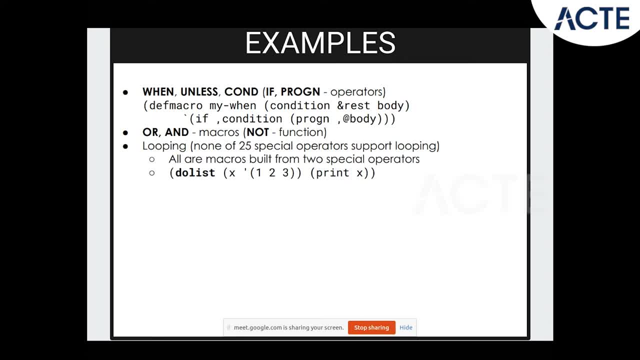 So or, and and are macros, And not is a function. All right, So we will have a look at it. And looping is none. So those 25 special operators, none of them support looping. Okay, They only support if, and if is a special operator. 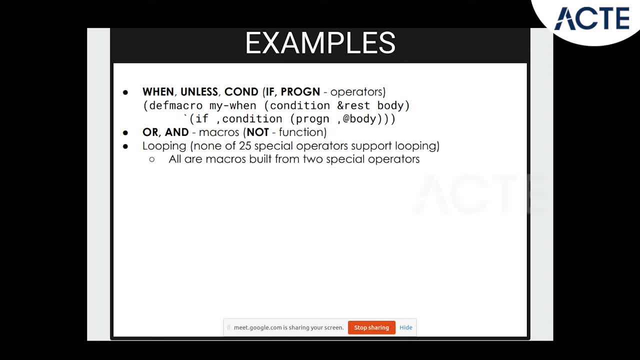 But the other operators, none of them support actual looping. All right, So they have but kind of a go to Some go to thing that they said. So there is some small low level stuff for branching, But it does not have any any loop as a special operator. 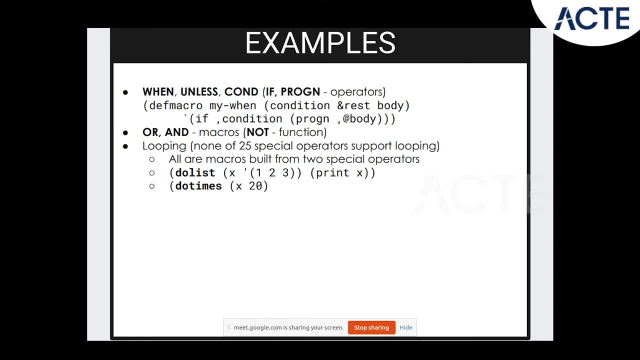 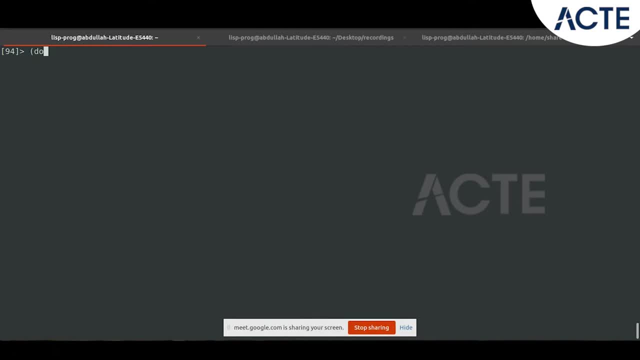 All are macros. So we had a look at this. do list, Do list. we did not have a look at it, So I can just show you how do list works. It is very neat thing. Of course, nowadays we have this in many programming languages. 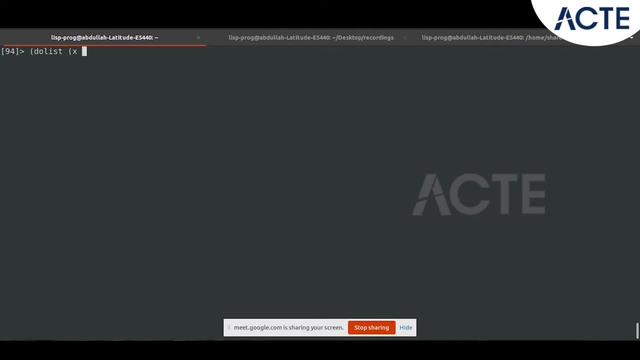 But yeah, It is probably the first to come up with this type of thing And it is very straight forward to do it Here. So the thing to notice that there is a macro- Okay, Actually, it iterates over all the elements in the list. 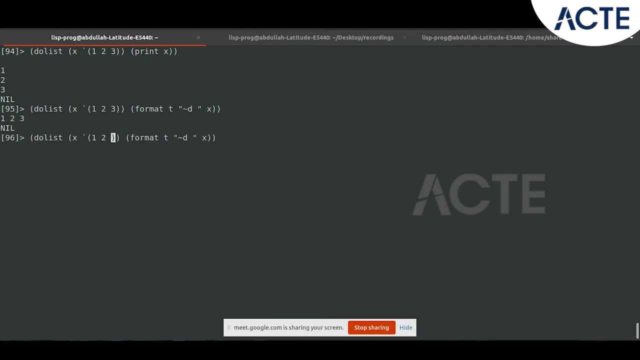 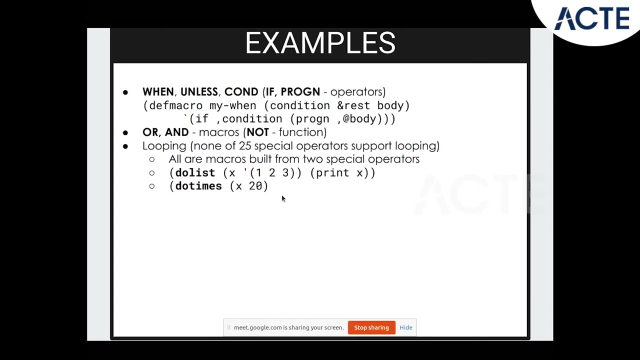 It is still not work because of this thing. So any doubts here so far. So do list is one construct, Okay, And similarly you have do times, which we had a look at it yesterday. Just look at this, Okay. 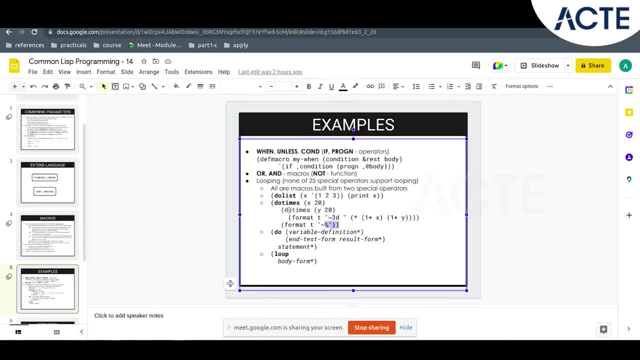 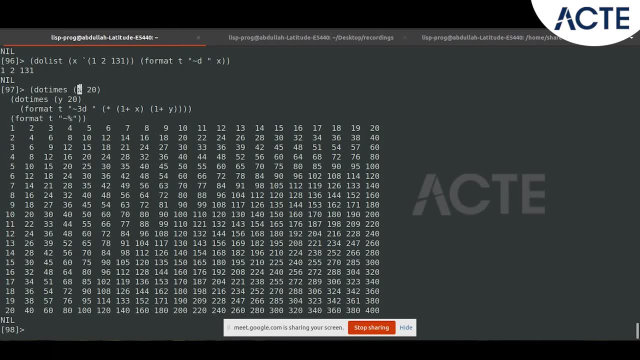 This is very interesting The way it does it, And of course, we have had a look at do times, Okay, But a nice example is given here, Okay, So what happens here is x is going from 0 to 20.. 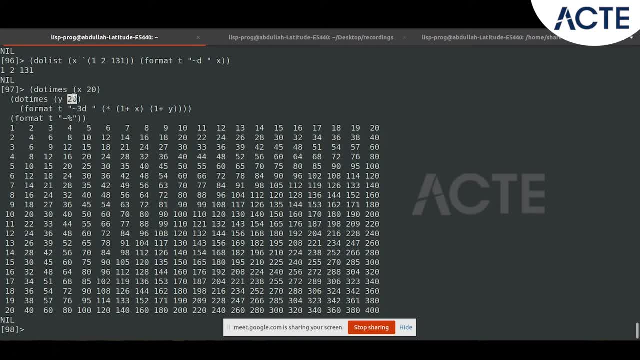 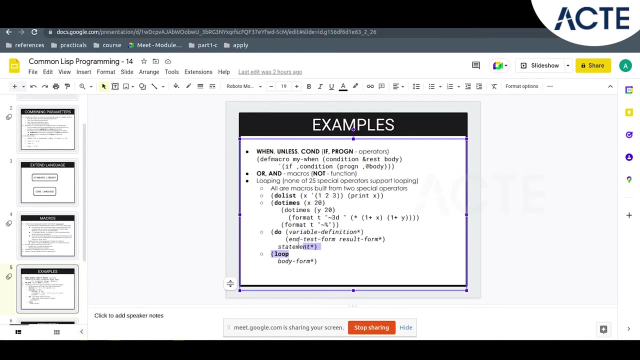 Y is also going from 0 to 20.. So you just loop as long as it hits the thing. So do list and do times are two macros. Okay, They are two macros And they in turn call another macro. So it is like two levels of definition. which is a do variable? 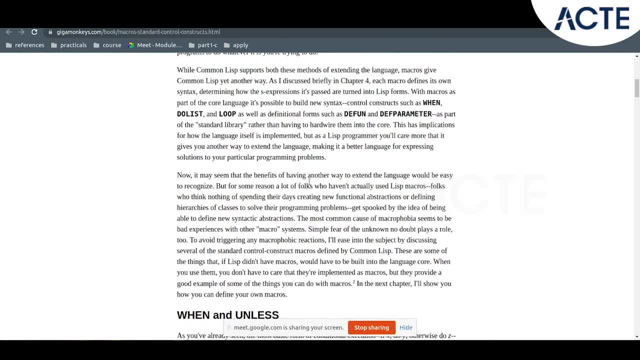 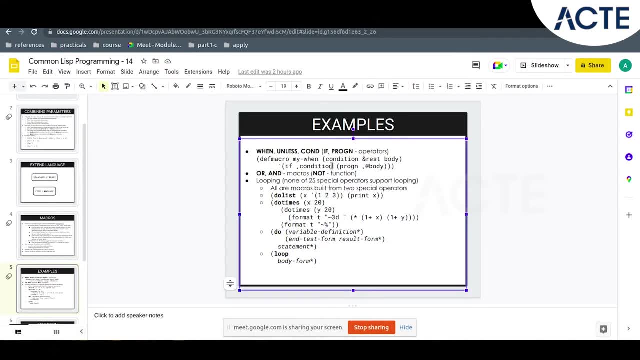 So you can see here he is saying that you know, yeah, so let me, just before we go to do, let us, so that is do and that is do. we will come to do and do. we will just have a look at what is this when? just a motivational macro. what is this when and unless? all right, 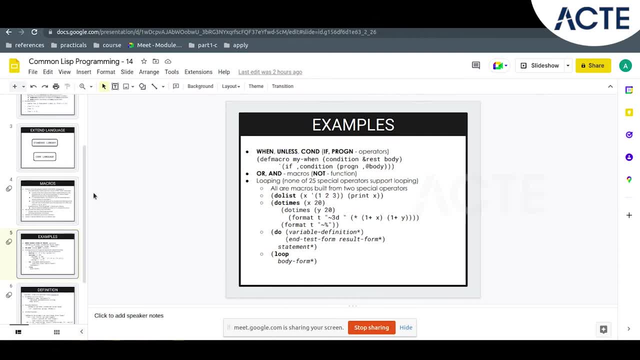 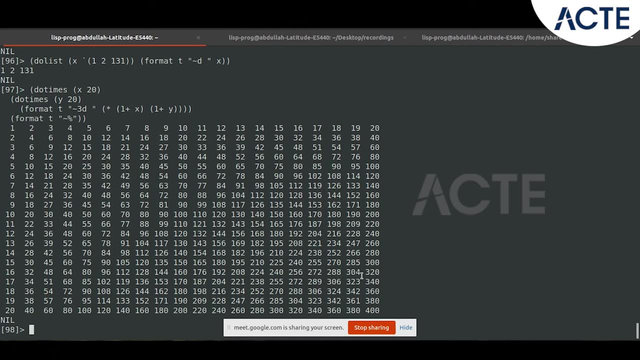 let us just have a look at it in a bit more detail so that we can- yeah, we can, we can- understand the macros a bit better, okay, So I mean the motivation for having macros. one example of it. So, for example, what happens is: so this is clear, right? I hope this thing is clear. 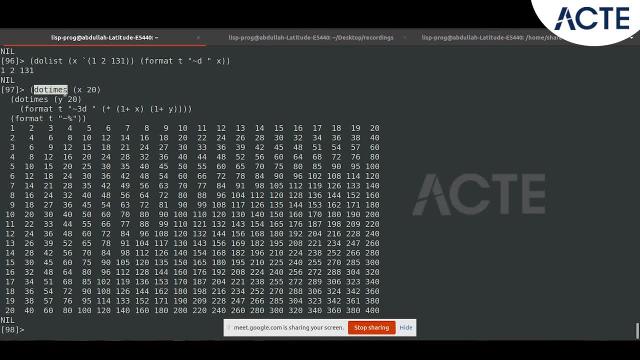 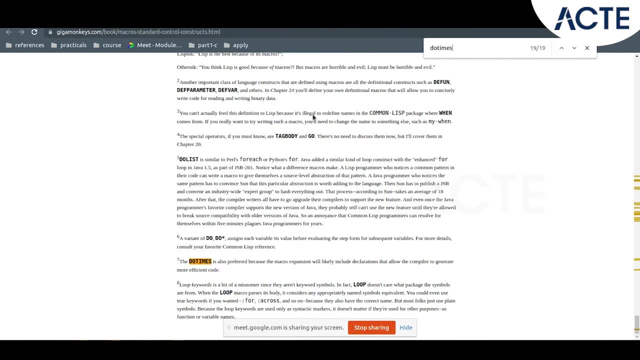 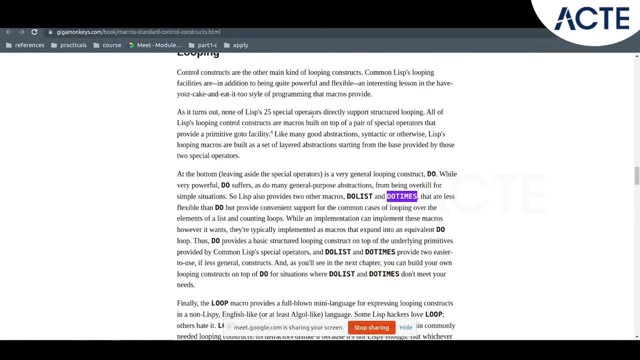 how this is getting generated and yeah, so do times is. I just wanted to see one more thing: So do times is actually built on. it translates into: Okay, So, yeah, so the implementation can implement these macros as it is. okay because it is. 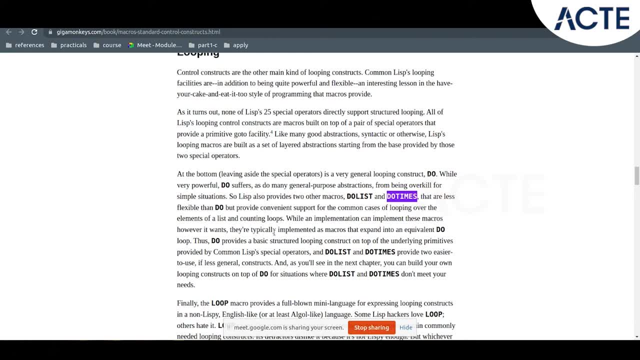 built over the core language. all right. they typically implement it as macros, Typical implementations like common list, I think. I guess the C list, what you are using, will have the same approach. they are implemented as macros that expand into an equivalent do. 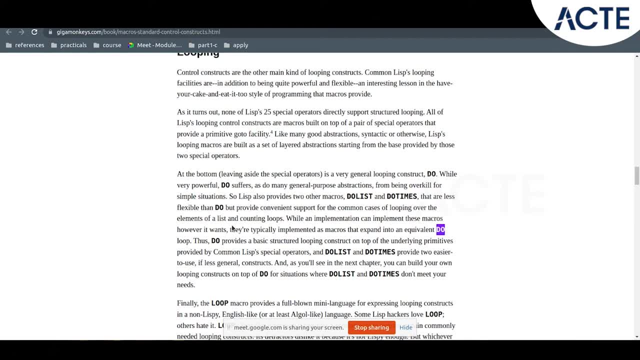 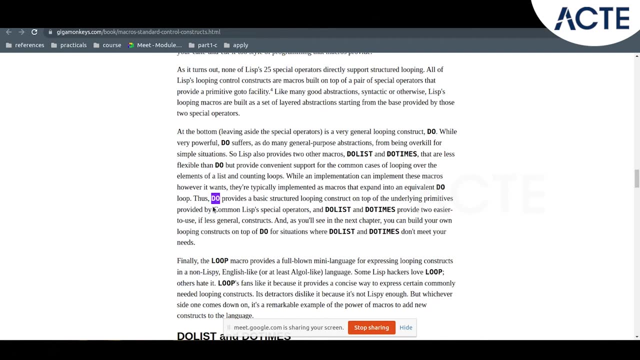 loop. So this do list and do times will translate into do and do is much more. I think it provides some more features. okay, in a very succinct manner, and it is also very difficult to get things right as we will have a look at it. I would like to show an example on that today. 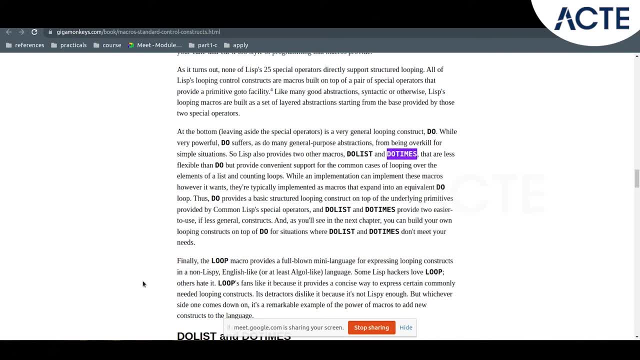 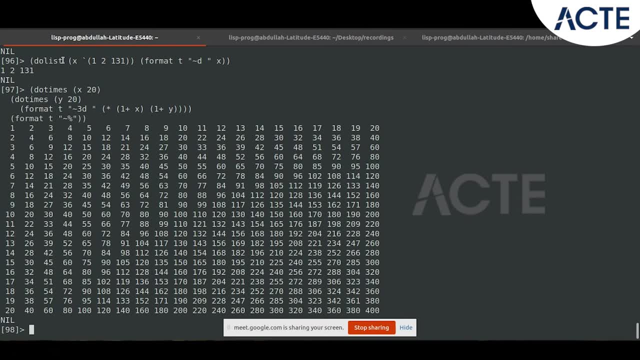 itself. But basically what happens is do list and do times is some kind of simplification over do. All right, do list and do times. they simplify your because sometimes you might, this might be enough for you. Either you want to loop over a list or you want to go like iterate over up to some value. 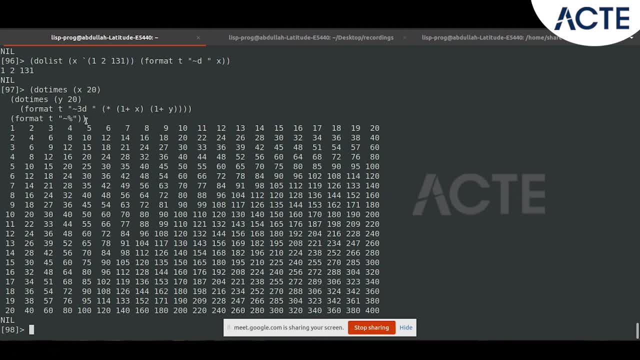 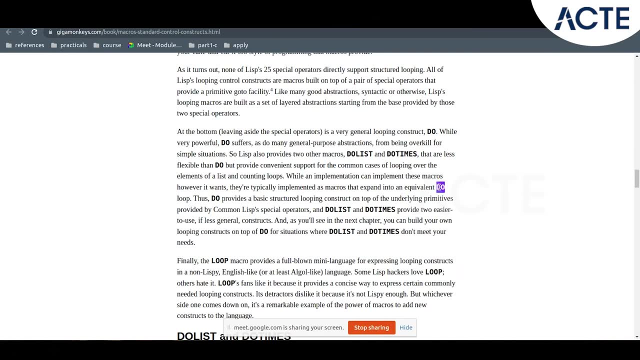 integer. So you have this thing and it is a macro. So macro it gets translated into do, and do is also not a special operator, it is also a macro. So you have these multiple nesting of macros. One macro gets translated into another macro. 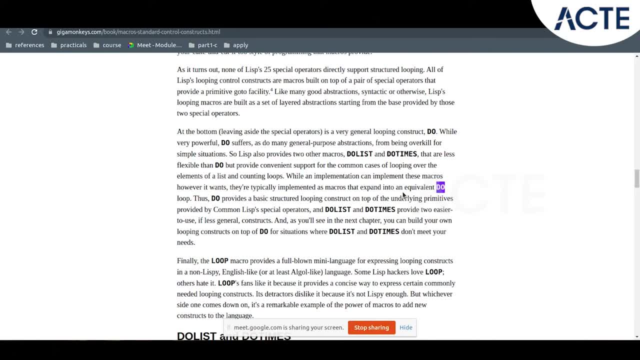 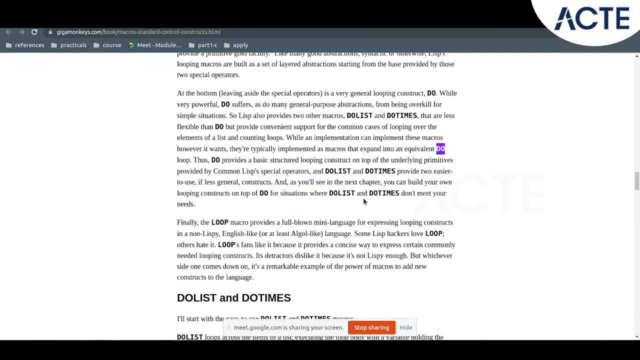 Another macro gets translated into the actual code, which will be a special operator or function, call Clear. So this is the scenario here, and we also have something called loop, a loop macro. I will just give a short thing as to what this when is okay. 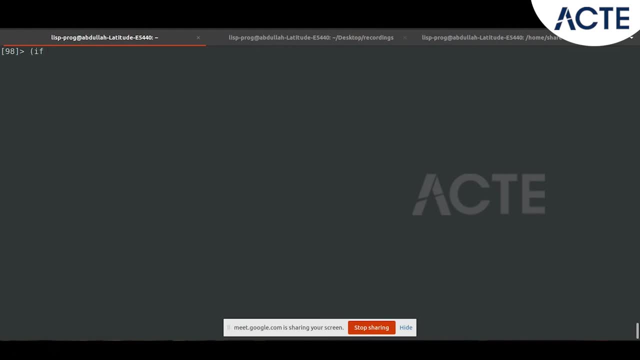 So if I have to have going back to if, if I put a condition right, if I put if greater than 1x, let us say y, okay, So we had this thing right In fact, Yeah, So if I, if I- let us just take the example that we have here, let us not create an example. 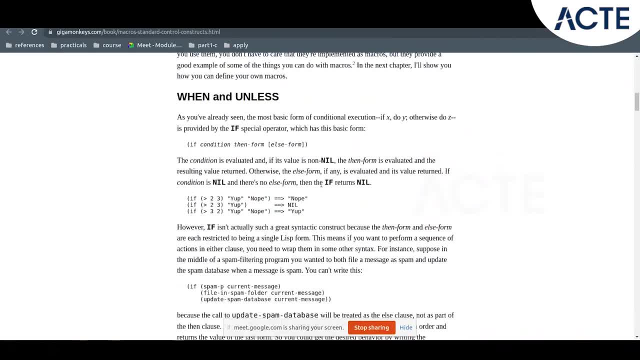 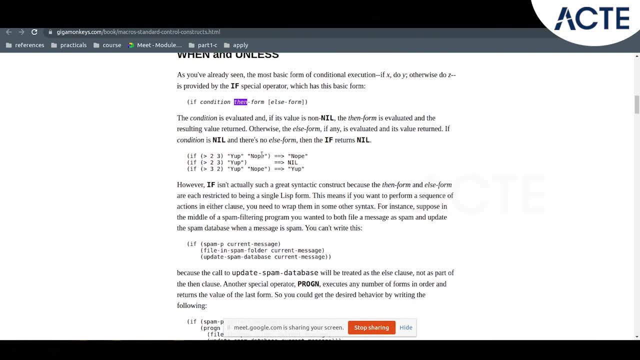 Let us just go with the example they have. So if condition, then form, else form. you saw that how right. sometimes you do not want the else form, Okay, It is like this. So, for example, spam is what he is saying. 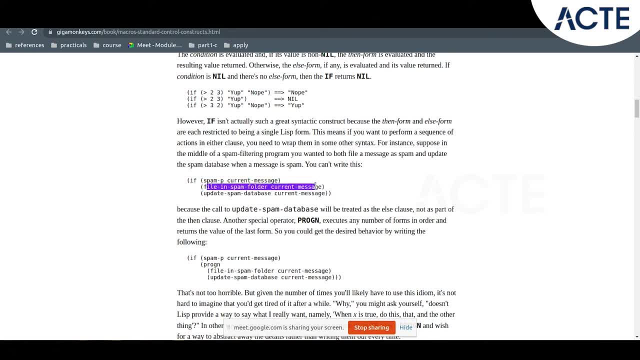 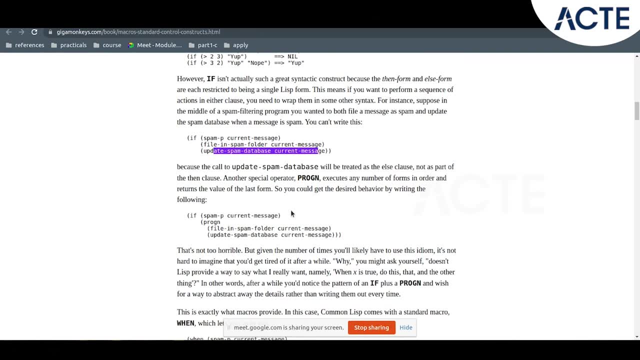 If the current message is a spam right, You want to do something, You want to file in the spam, update the spam database and current message and you want to do some processing. There is no else part. Okay, If there is no else part, how do you go about doing it? 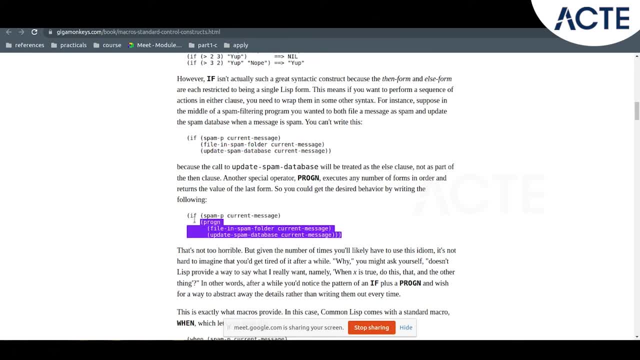 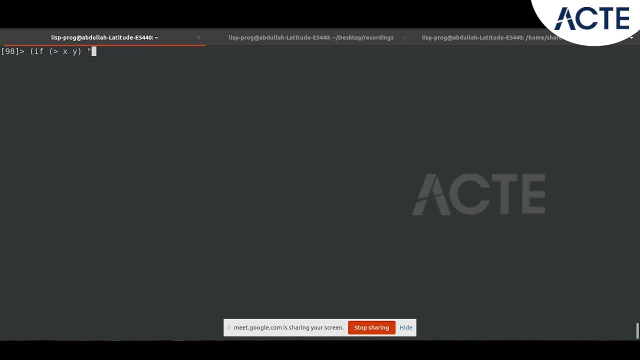 We will have to put in a progn. You have to encapsulate that in a progn and say: do these set of instructions? Okay, But get it. So let us say I want to print in like this: Hello. I will say hello. 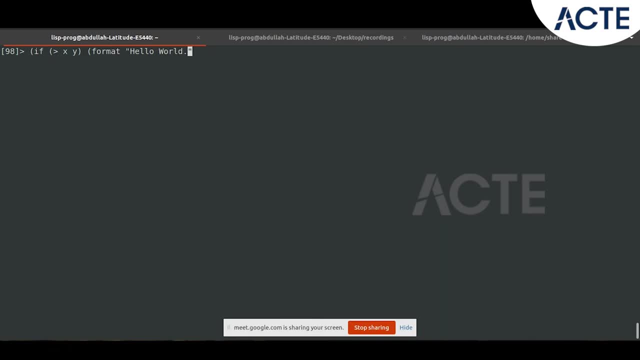 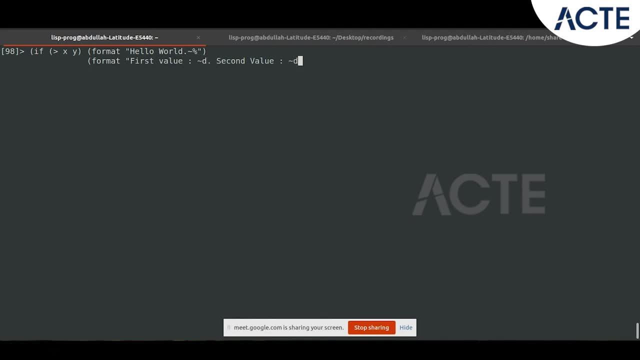 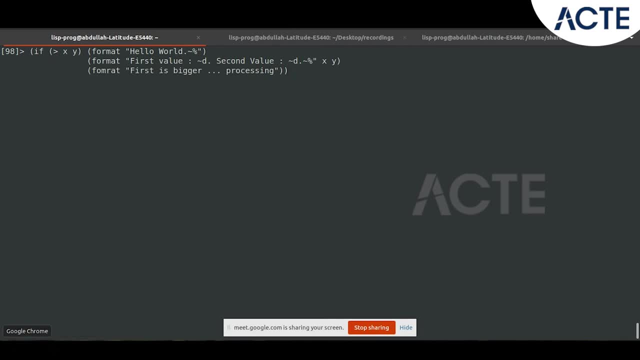 else part. will this thing work? because I don't have an else part, all right, no else part, and I want to write a body form star. will this thing work? the problem with this? there is a problem with this, okay, and there are. yeah, you can see it in two ways, okay. 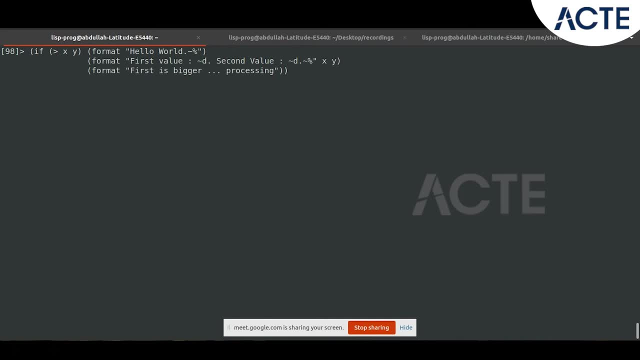 first of all I need to define it. of course, x and y are not defined, all right, so too many parameters. so I will define x and y. x is 1, 0, 1, 9,, y is 1, 5, 5,, so 19. 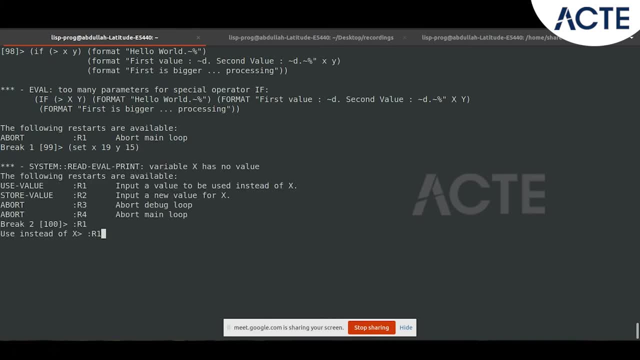 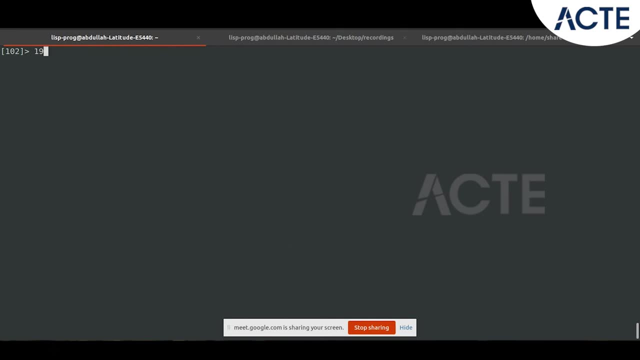 is given for 2.. Let's say we have just two forms, okay, now. the issue with this is basically that: yeah, so okay now. I have only two lines. now what? all right? so let's say we have just two. 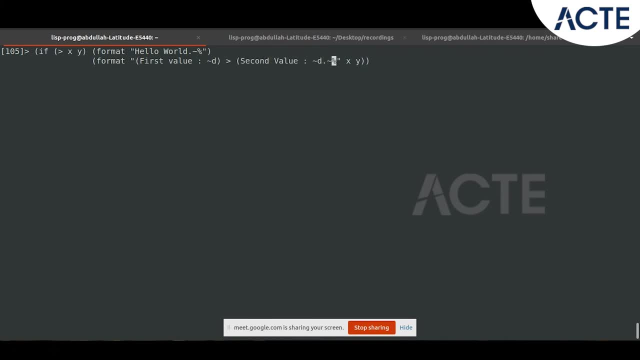 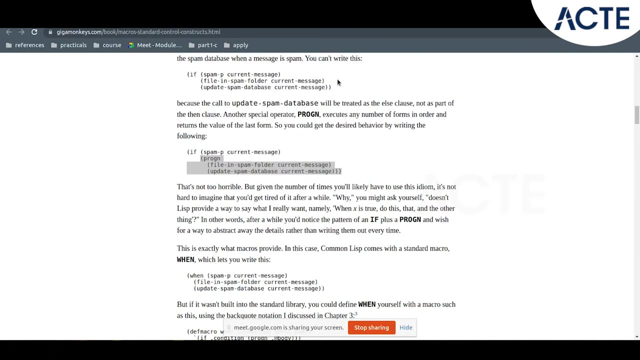 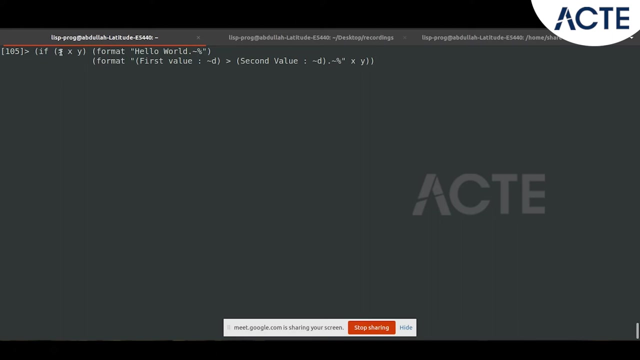 lines. okay, All right. All right, I have only two lines, but, and what I wanted to like, the spam message, right, if it is spam, I want to do a series of instructions. okay, so, if I have this, so I have put in. 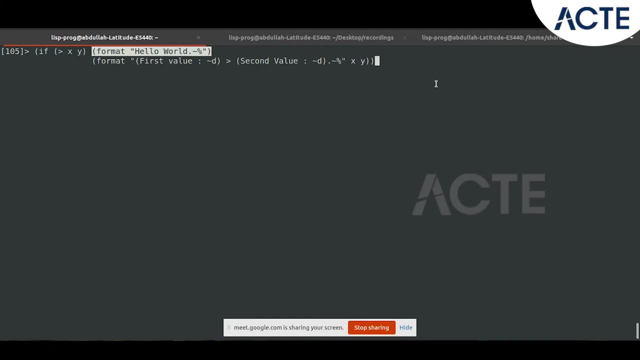 the format. of course, third line was an issue, so second line: what will happen now? the semantics is different now. okay, now the this, I wanted to this to be a part of this thing, All right, So this will not work because, okay, this will not work because of: okay, hello world. 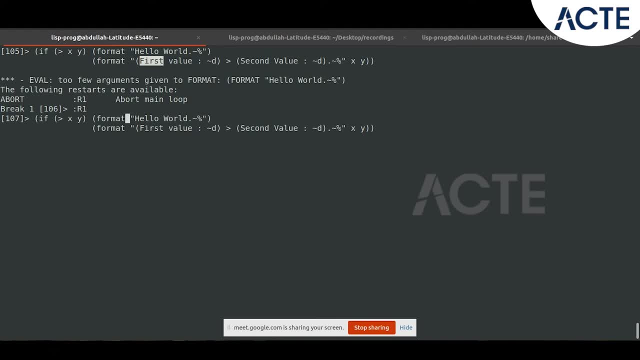 and format t, so that I was missing here. all right, so it is syntactically correct. the program is syntactically correct, but what I wanted is I wanted this to be a part of that greater than so. in order to do that, what I have to do, I have to write it like: 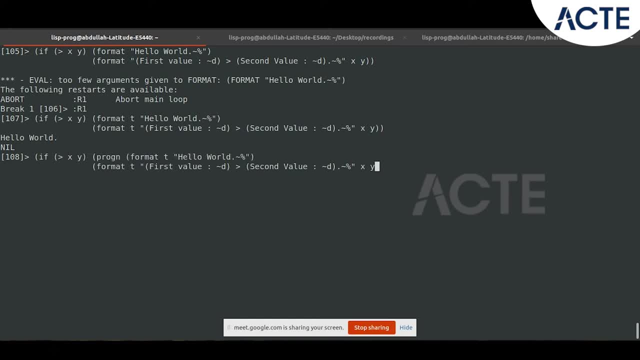 this All right, And close this, close that and close that. So this is what I wanted. okay, else part, I do not care. let us say I do not have else part Now, even if I have to, just for the. you know, I know, I know I do not need an else part. 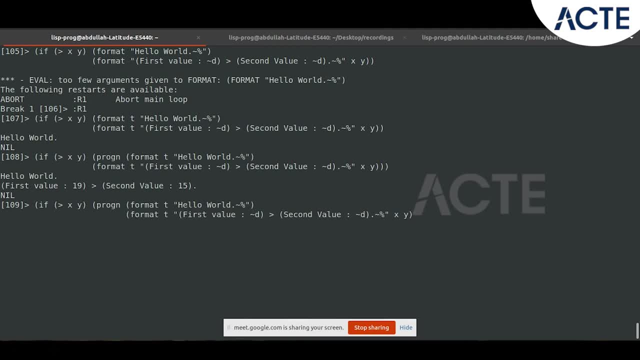 all right. so just a motivation for one example where macros really help. okay, the point of having a macro. So why do I need this thing? right? why should I have to define a progn? progn is a little bit, I mean. every time I have to define it, I have to, you know, match the parenthesis like: 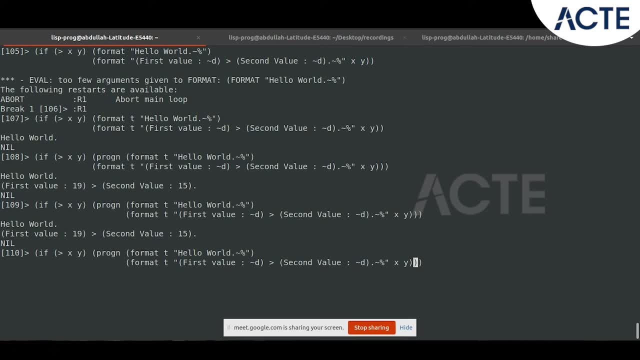 this another extra unnecessary bracket for progn. okay, so what does when do when does the same thing. I will just give you the motivation for when. this is the motivation for when and it is also motivation for why you might need a- one of the advantages of having a macro thing. 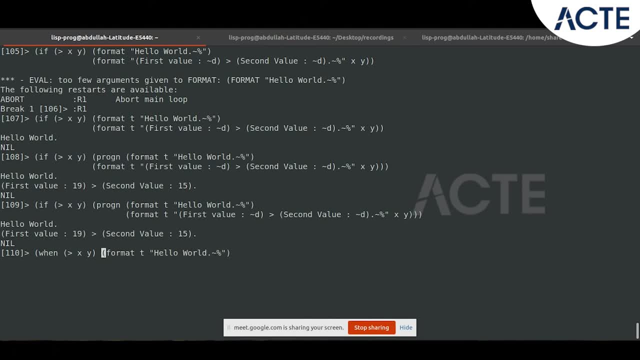 So something that you are regularly typing in, you can save yourself some amount of typing. you do not have to put in the brackets. now You can actually do it this way. So you have a new thing called when, construct called when, and you can actually do this thing. 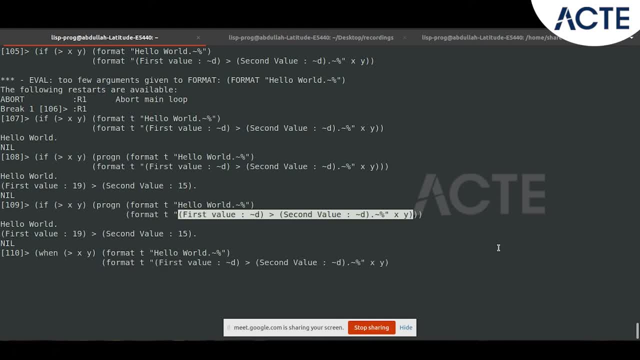 the same thing without one extra command and one extra parenthesis. So to simplify your programming thing, programming some stuff so you get it right. I hope the when thing is clear and in fact the when is actually a macro which translates into: if 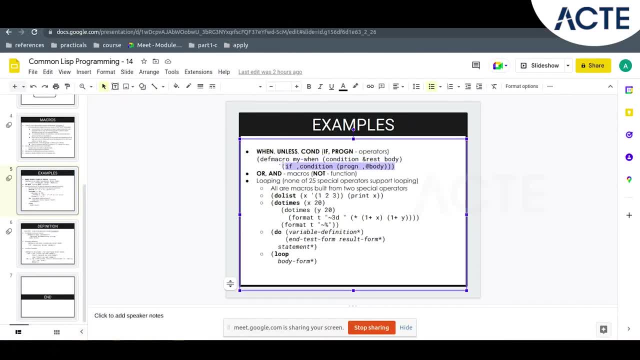 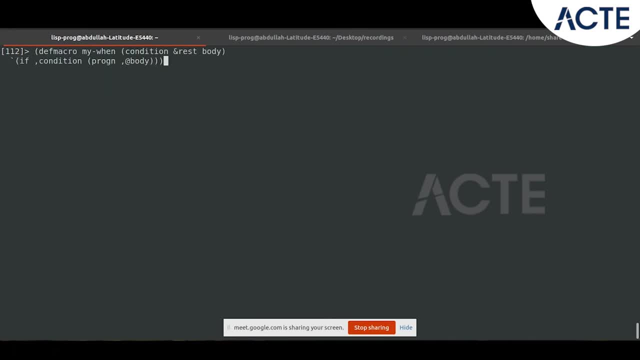 So here is one example of defining a macro also. so I am giving you a macro definition. So this is how you go about defining a macro. So you say my, now I am using my when. you cannot use when, because it is already defined. 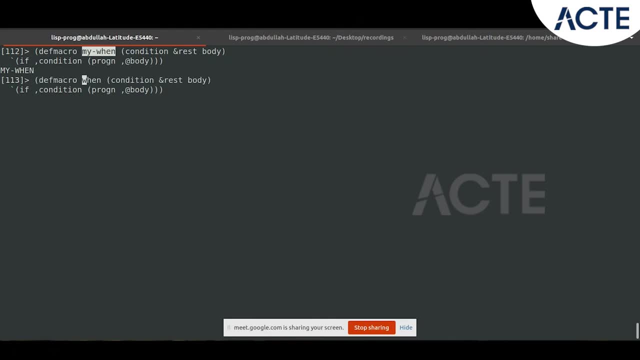 It is a system thing and it will throw in an error: special operator and may not be defined. So it is saying special operator, but it is not actually a special operator, it is a macro. So maybe it is a special operator here, I do not know. but even if it is not a special, 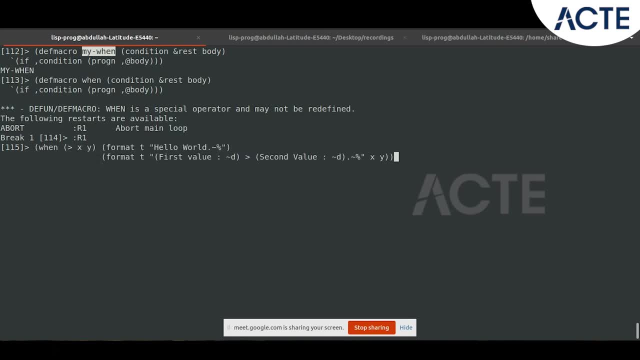 operator. you can define it like my when you saw the point. So I can have my own control construct which does that one thing. So the when is it seems he is saying it is a special operator. I do not know whether 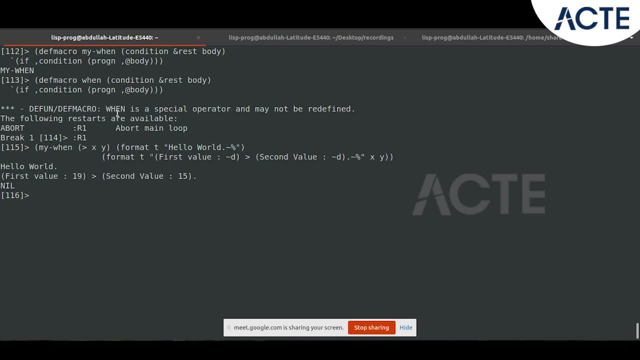 he means special operator or it means a macro, but let us ignore that. even whatever it is, we can actually define it in ourselves like this. The way to define it is this way, like this. So this gives you this other thing. so this is the back quote. we will come back to this. 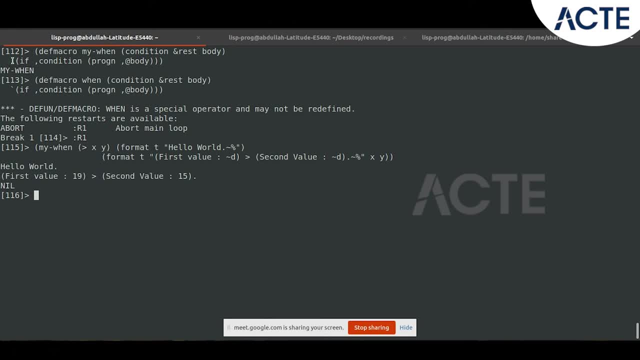 definition next class. we will have a look at detail into it. but it is a back quote and you can actually plug in the body. So instead of having to write every time if condition prog in, it is basically doing that for you behind the scene. 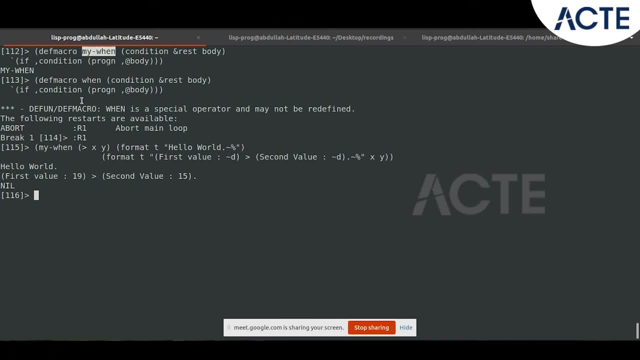 Basically, I have defined it for myself now: my when, My when, and I am using it as when. So this is the point of that and similarly you have. unless Unless would be like the opposite of that. Unless means that it is going to be like this: 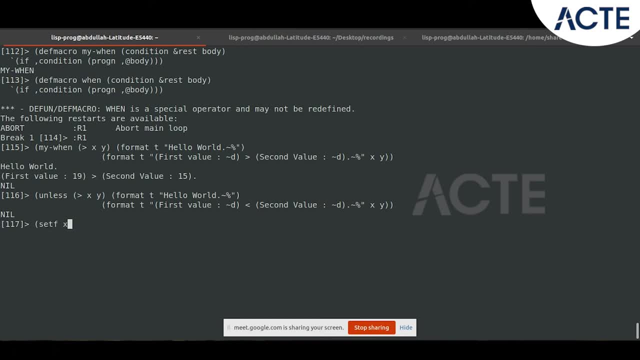 So now we have nil. Now let us just put set f x as 5.. Now you have the unless. the unless is similar to when, Only thing when the condition is false. it will go into that and it will give you the. 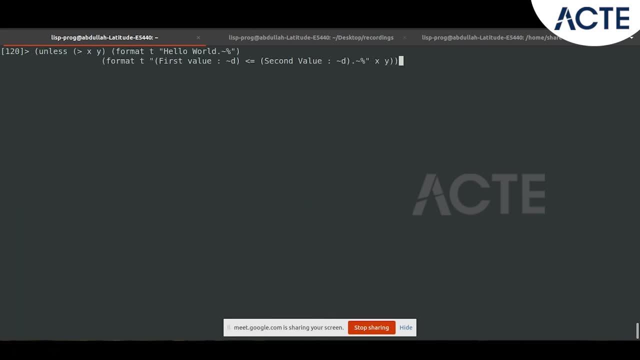 other thing. It is less than equal to, Unless greater than right. So I can say x as 15 and again this will get triggered. So you can see that it is. if it goes 16, it will not get triggered. So it is basically. it helps you to write. I hope you see the power of macros here And macro defining macro. the only thing you need to know is that there is this: the back quote is the important thing, and this is at the rate of- and we have other some. 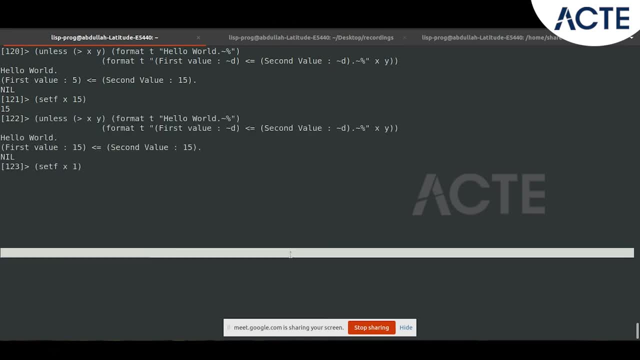 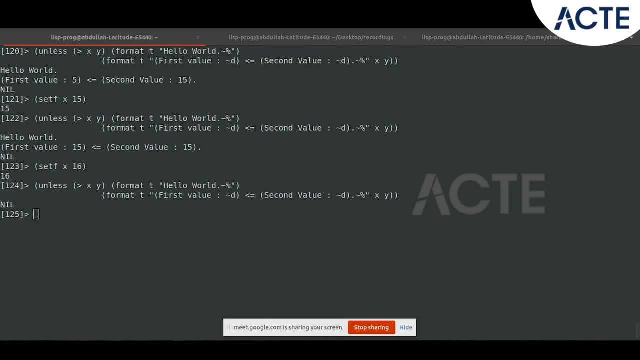 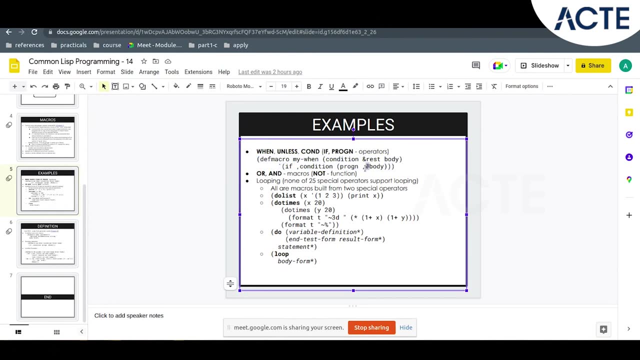 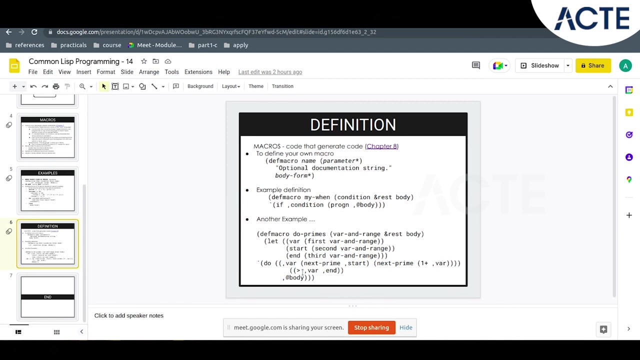 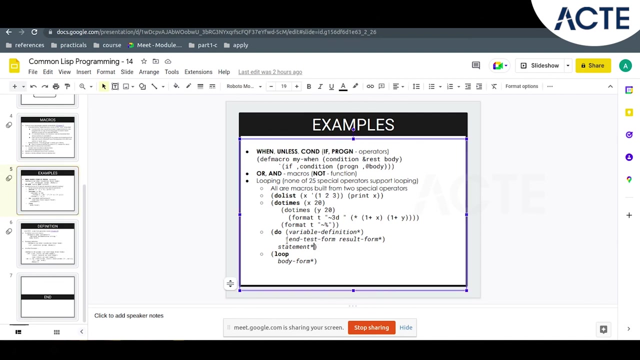 So, let us see So, let us see, So, let us see So. for example, this is one definition: all right, Do is something you said it didn't go Do. We will do a do and loop tomorrow. 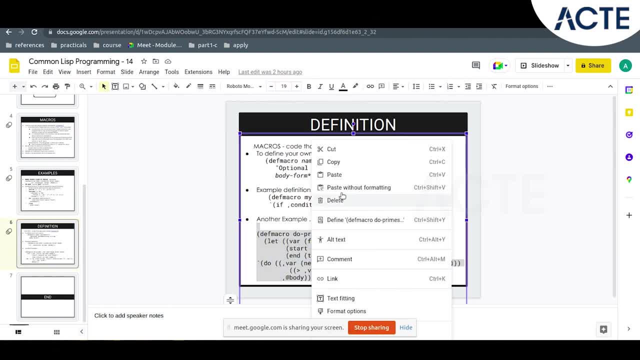 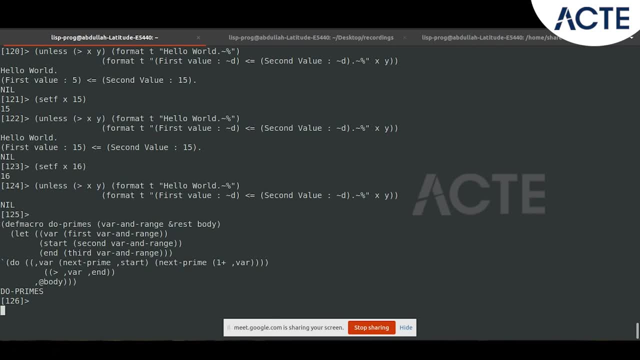 And we will also have a look at this function. all right, So let me just give you an example of another macro. Like: what does it take to build your macro of your own? This is my own macro is given in the exercise also. 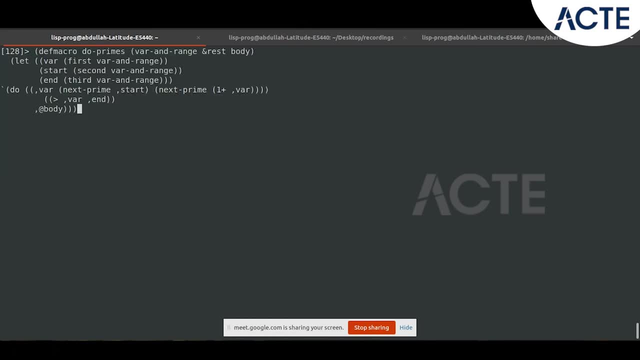 I mean in the book, given in the book. So what it is doing is it is translating that. I will discuss 2 tomorrow because it is time up. 2 is little bit involved, But basically, you see this special characters is back quote, comma and at the rate of comma, at the rate of. So these are the, so you. 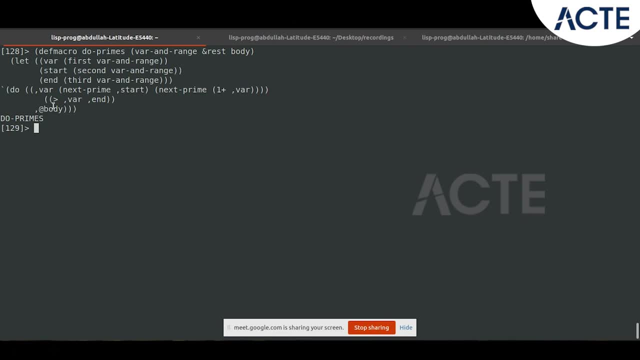 are giving the program itself as this thing, You are giving a let form, So def macro. basically, what it does is it is like def1, just like def1.. You define the, you give the name, you give the parameters and again parameters could be required, optional and rest. So here it. 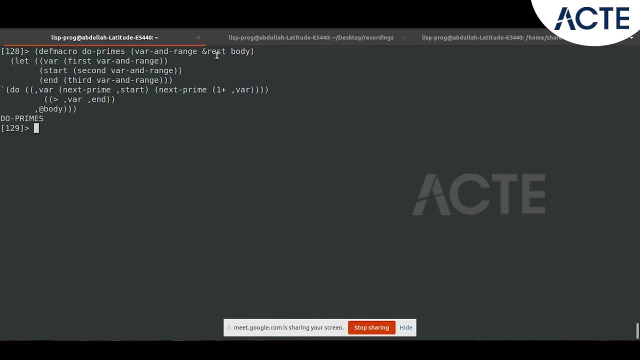 is saying rest. Most of the time you will be using required and rest or required and optional. Very rarely you will be using other things, But it is good to know. and keywords also. You can use keywords in some way. it has some sort of benefit of using keywords. 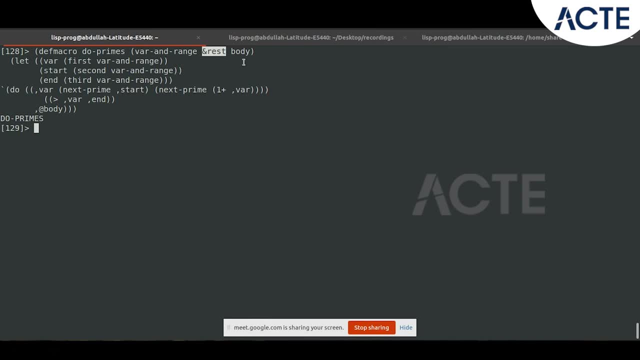 But yeah, you will have one or more of them. I mean required and optional, So you can use different kinds of keywords as required, plus one or one other form. So you can just keep that in mind. And then there is let form. Let is also proper. you can, you can add functions into your macros.